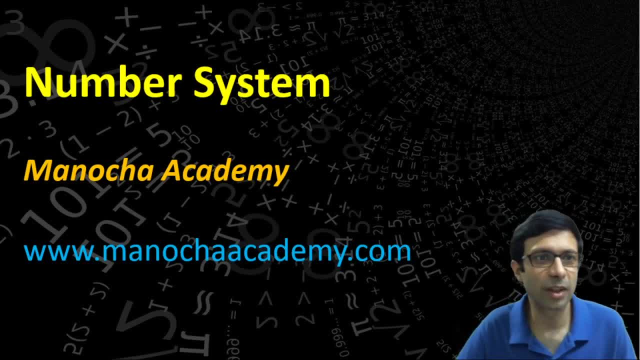 Hi friends, good evening. So I see a lot of folks are out here. Can everyone hear me? So welcome to this class on number systems. Yeah, good evening, Hi, good evening, Satyam, Hi Manoj Hi Prabhakar, Hi Renu Hi Vinita. Good evening everyone. So this is a really important topic in mathematics- the number systems, And we'll be talking about rational and irrational. 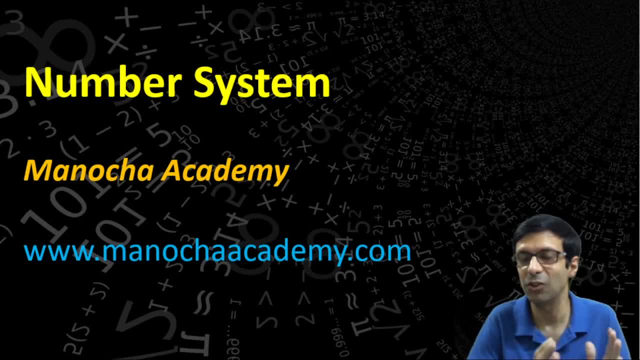 So we'll be talking about the real numbers which can be divided as rational and irrational, And this class is really important for class 9, 10, even for class 7 and 8.. So if you're from class 7 to 10, this is a really important topic for you to understand And I'm going to make the concepts really clear and easy for you. So I'm sure you'll be a master of number system after watching this class. 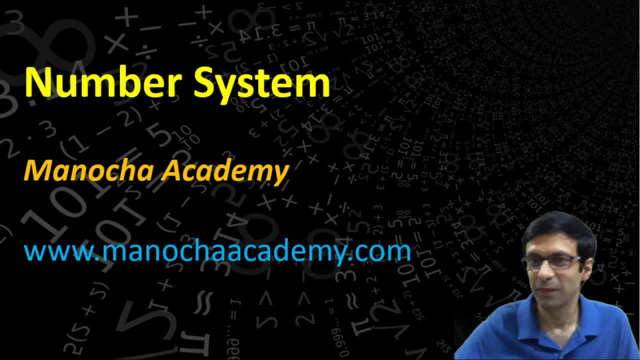 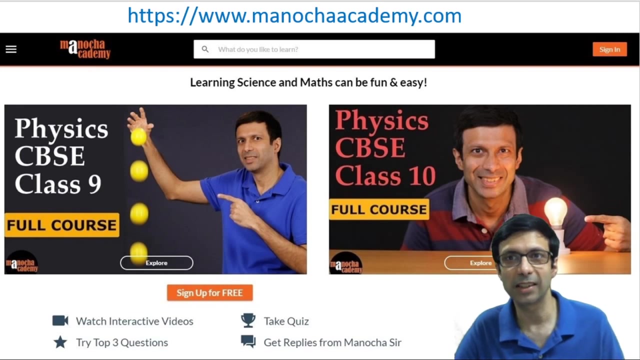 Hi, good evening. So I can see a lot of folks are out here: Hi Ayush, Hi Anuj, Hi Sreenivas, Good evening everyone. So welcome to this class on number system. So this is our maths class And, guys, if you haven't checked out the website manochacademycom, do check it out. So we have these physics, class 9 and class 10 full courses And soon we'll be launching the chemistry and math courses also on the website. 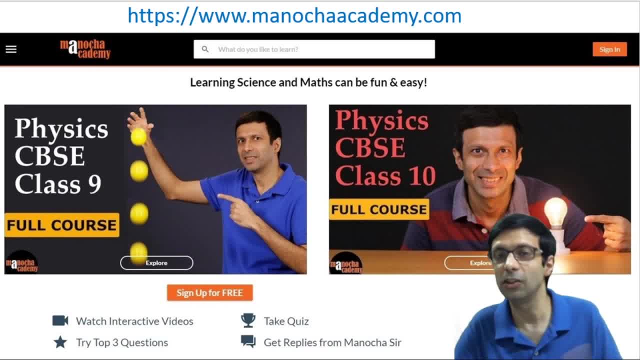 So, if you guys haven't checked out these classes, these courses, do check it out. we have interactive videos, quizzes and questions for you to practice, so these courses will really help you in your preparation, and we have big discounts going on on these courses, all right, so, guys, let's. 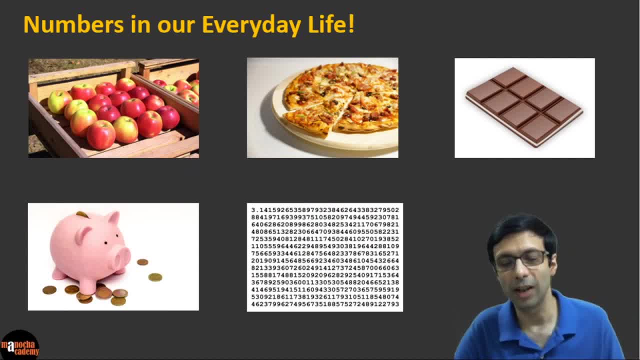 get started with this amazing maths topic on number systems. and we see numbers in our everyday life, right? so, for example, when you go to the vegetable shop, let's say you want to get a dozen apples. so let's say you want to buy 12 apples, right, so that's the number 12. or let's say if you're eating: 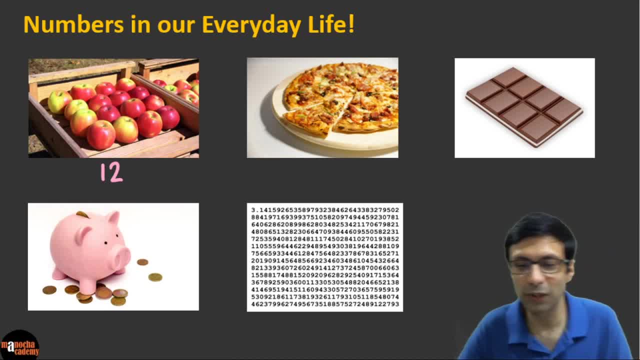 this pizza. so if you're eating one slice of this pizza, we can say you had one sixth of the pizza, right? so you can see there's six slices, and if you have eaten one, you've had one sixth. so that's a fraction number, right? and let's say you 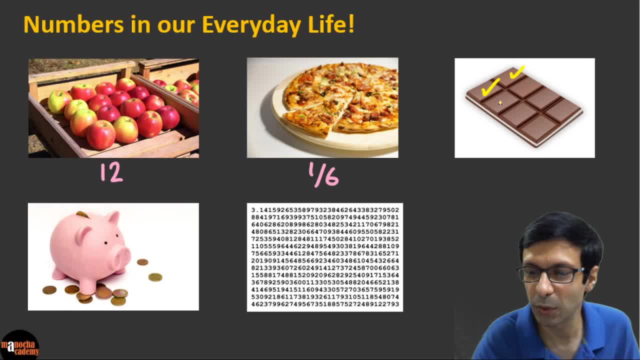 eat three pieces in this chocolate bar. so this one, this one and this one, right? so how many chocolates have you eaten? how much chocolate have you eaten here? we can see that there are eight pieces. so you've eaten three by eight, right? so you've eaten three by eight of the chocolate. so that's a fraction, and let's say this is: 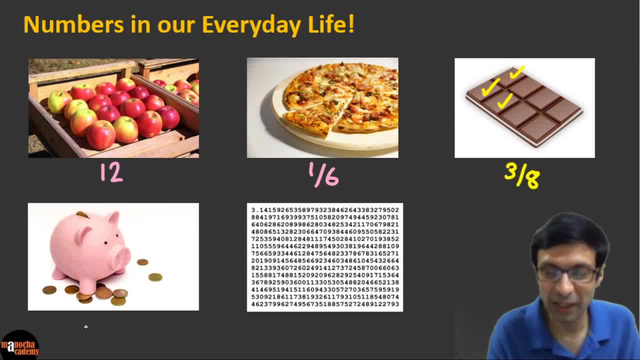 your piggy bank here. okay, and let's say you've saved 21.50 rupees in your piggy bank, so that's a decimal number, right- 21.5. and guys, can you tell me what is this big? And guys, can you tell me what is this big pie? 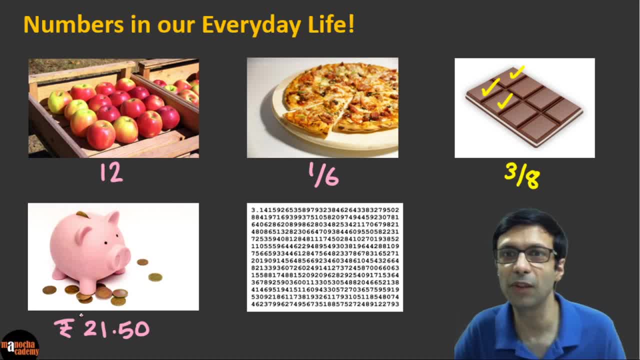 number that you see here: 3.14159265 and so on. so, guys, can you recognize the number in this picture here? so I'm talking about this picture. so what number is this? very good, I see a lot of you are giving the answer. it's. 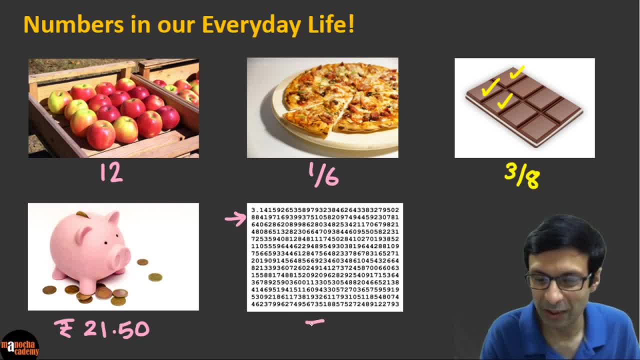 the value of pi. excellent, so this number is also very important number in maths. you've seen it: the it's the value of pi. so we see numbers all the time in our everyday life. excellent, a lot of you have got the number pi and these numbers are really important for us and, as you can see, there are different types of 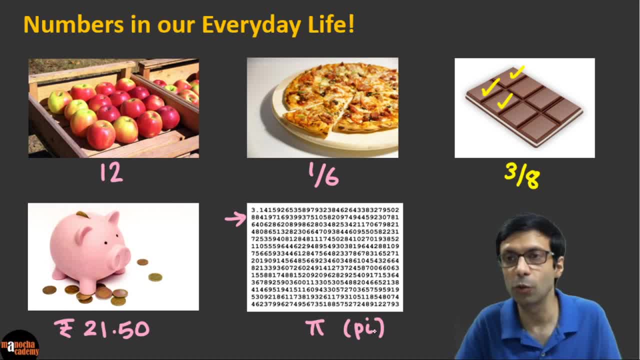 numbers. so we have, like: you went to buy apples and you wanted to buy 12 apples, that's a integer number. then you have 1 by 6, 3 by 8, fraction, then you have a decimal number, then you have numbers like pi, since we have so many different. 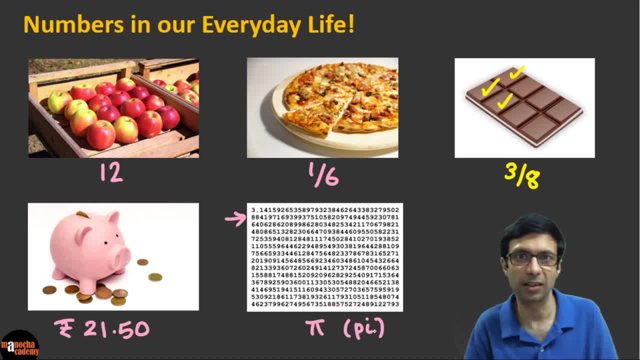 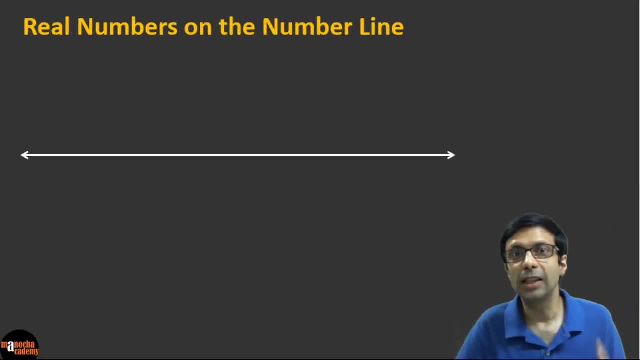 types of numbers. so we are going to organize the numbers in this class, right, and we are going to talk about the different type of numbers. okay guys, so let's see. so let's start with the topic. so you must have heard of this term. it's called real numbers, right? so we are. 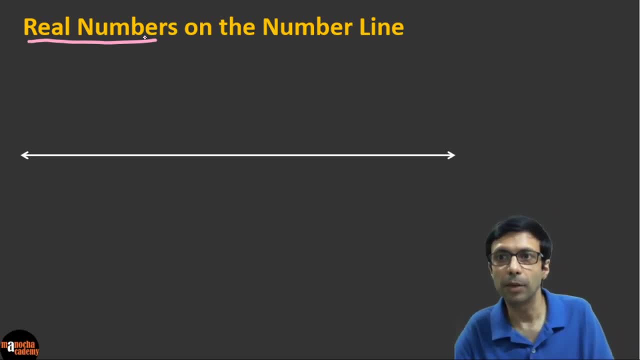 going to talk about. what are real numbers? real numbers are those numbers that can be represented on a number line. so let's start with a example. so I'm sure you know that these counting numbers, like one, two, three, three, four and so on, these can be represented on the number line. so can 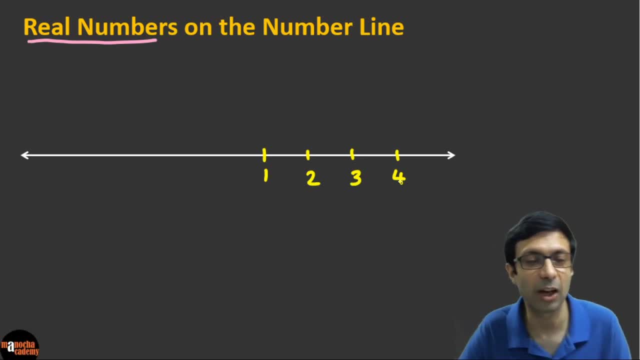 you tell me, what are these numbers: one, two, three, four, these counting numbers known as: so guys, what are the numbers that I've represented here on the number line known as one, two, three, four and so on? right, someone says integers. good, you're saying real numbers, yes, natural numbers, excellent, so actually all your. 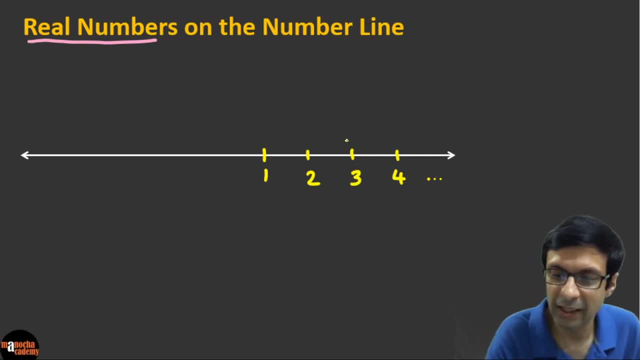 answers are correct. right, but first let's say that these numbers are called natural numbers. let's start with the simple case. so, as you can see, the numbers are marked here are called natural numbers. so which are the numbers from one, two, three, four and so on? right now, if we add the number, 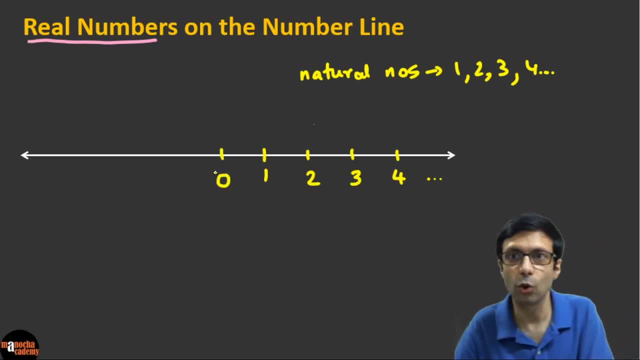 zero here, right then, what is this set? known as zero one, two, three, four. so zero one, two, three, four, guys, what is it called? so you must be knowing this. these are called whole numbers, right? so once you add the zero, so once you have zero one, two, three and so on, these are called whole numbers. excellent, I see lot of you. 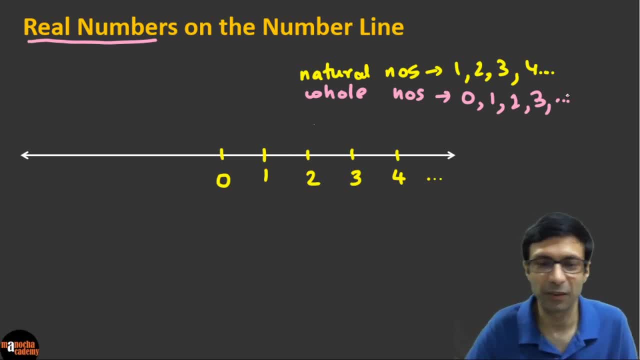 have written all numbers here super right and now you can. so we have the natural numbers here and if you add zero together, these guys are called whole numbers. and we can also add these negative numbers here, like minus one minus two, minus three, minus four and so on, right on this number line. so I'm 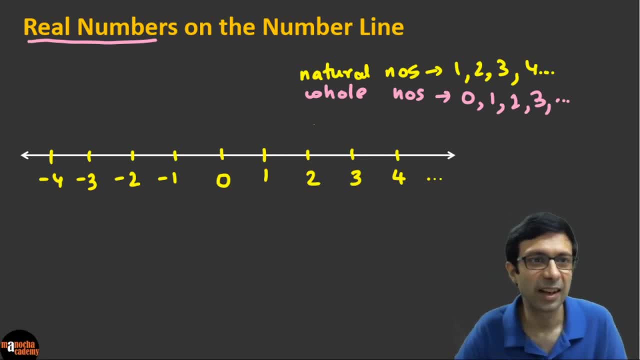 adding these numbers on the number line. so what is this whole set known as excellent? I see, you guys are amazing. I see the correct answer there in the chat. so these are called integers, right? so when we talk about these negative numbers- 0, 1, 2, 3, so all of these together, these are known as integers, right? so this whole? 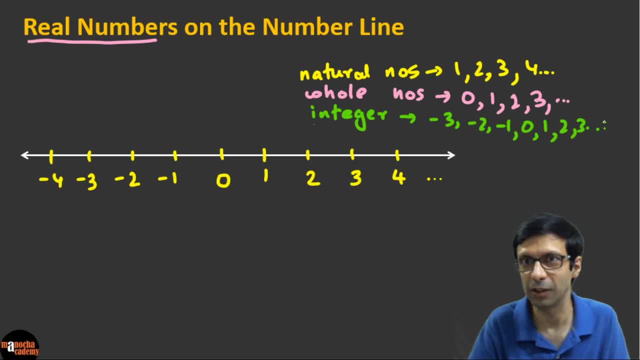 set here that we've shown on the number line is called integers, and whole numbers is the subset of the numbers from 0, 1, 2, 3, 4 and natural numbers, you know are one, two, three, four and so on. okay, so is this clear? that's great. 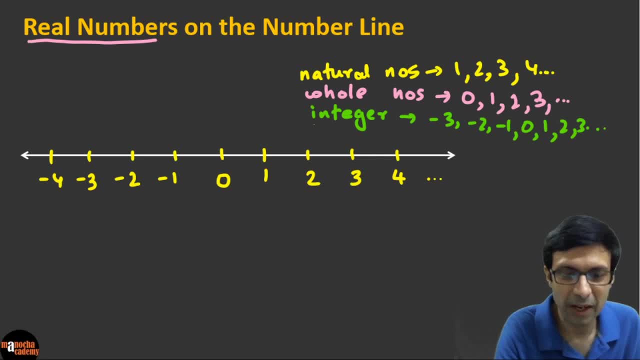 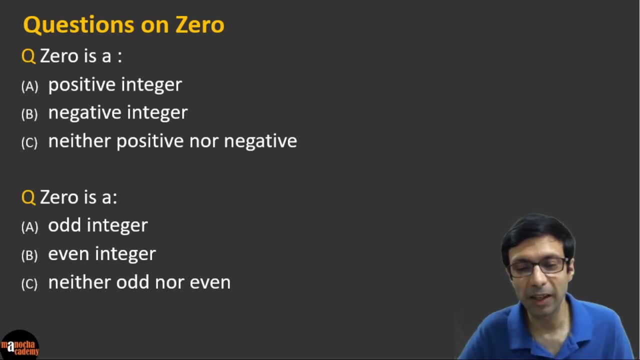 great, and now let's go ahead and let me ask you a question here. so let's talk about zero is a very important number, right? and so can you tell me? the first question is: is zero a positive integer, a negative integer, or is it neither positive nor negative? so what do you guys think from this? uh? 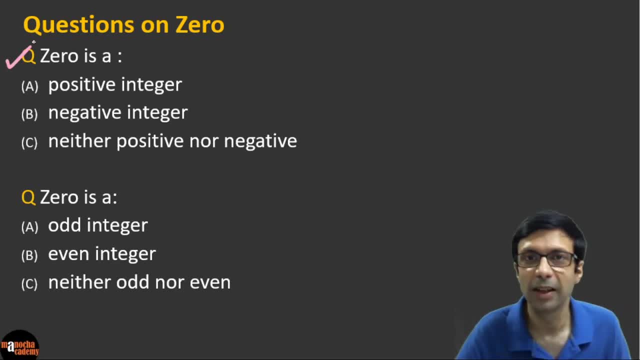 for the first question here. so i'm talking about this first question on top: is zero a positive integer, a negative integer, or is it the option c? neither positive nor negative. so i see a lot of you are saying it's the option c. excellent, that's the correct answer here. zero is neither positive. 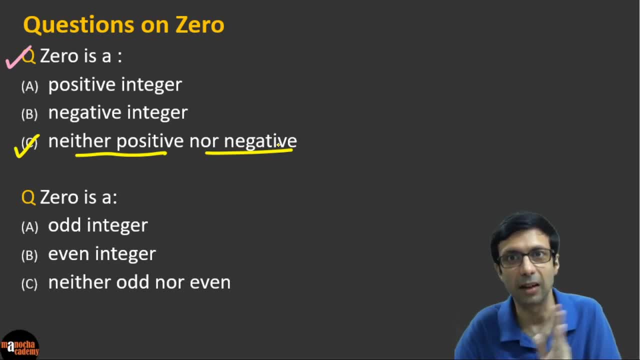 nor negative. okay guys, so zero is not considered either a positive number, nor is it a negative number. excellent, now let's take a look at the second question. so the second question here is: is zero an odd integer, g, are an even integer, or is it neither odd nor even? so what do you think here? 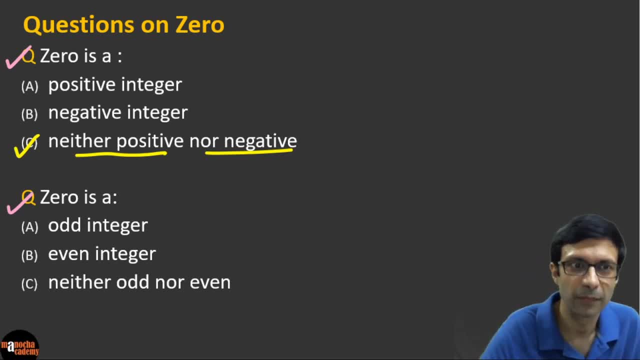 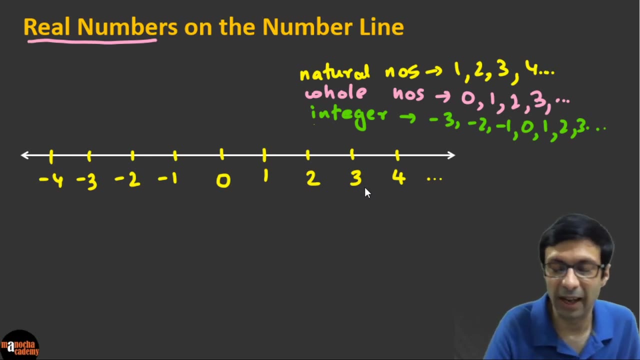 so, guys, what do you think is the answer here? so i see a lot of c's over here. somebody's saying b. okay, so you know the odd integers are. so if you look at this number line, the odd integers are 1, 3, 5 and so on. right and the even integers- all of you know they're uh, 2, 4 and 6.. but is 0 and. 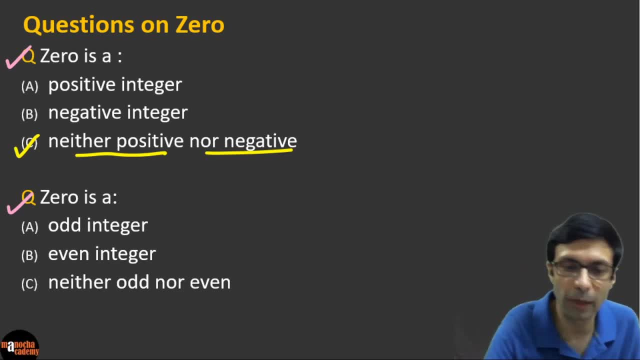 even an odd integer, integer or not? the answer is: 0 is normally considered an even integer, okay, guys. so 0 is considered, so B is the correct answer. that's very good. 0 is considered a even integer, okay, but it's neither positive nor negative. excellent. 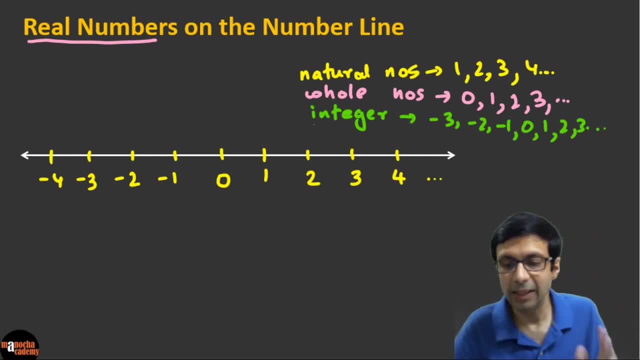 so now let's go back to our number line and, guys, can you tell me, are there any numbers between 0 & 1? so what do you think here? so the question is: can we have any numbers here between 0 & 1? what do you think? so, do numbers between 0 & 1? 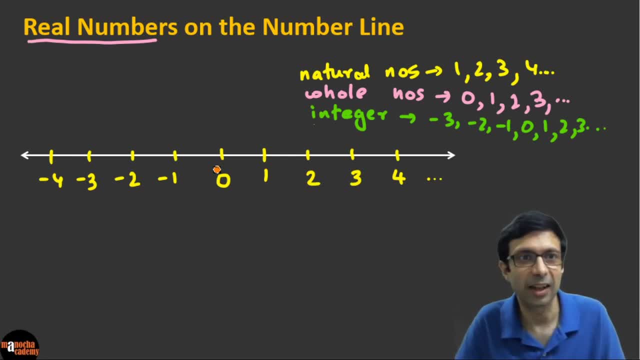 exist. very good. I'm seeing a lot of you are saying yes and you're saying these are called rational numbers. excellent. so let's take an example. so let's say, between 0 & 1, you can definitely have this number half right. so if you plot it exactly between 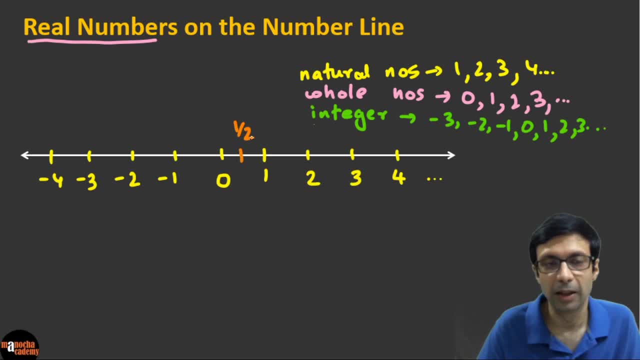 0 & 1, it's going to be the number half. similarly, if we consider numbers between 1 & 2, I can divide it into 10 parts, and if I mark the seventh part as 1.7. so right, so there exists numbers between these natural numbers, right, these are? 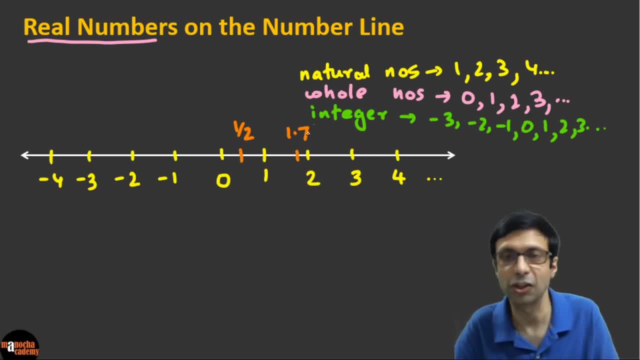 the decimal, decimal numbers or you can see the fractions here, right so, very good. so, as you can see, there definitely exists numbers on the number line between the natural numbers or between the integers here, right? so, for example, even between minus 2 & minus 3, we can. 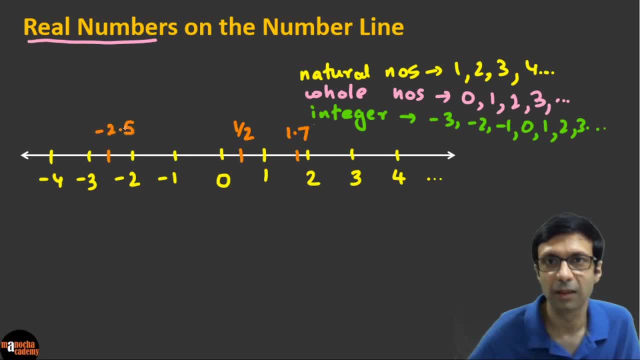 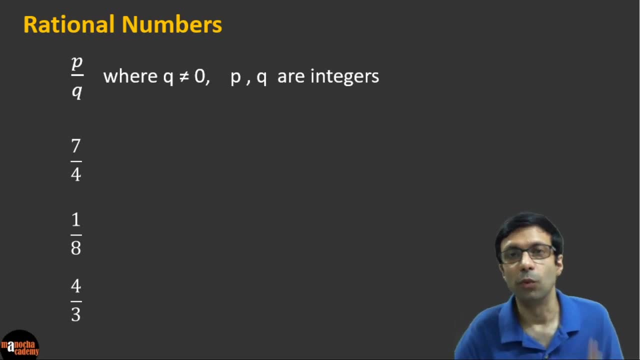 have minus 2.5, correct, okay, so let's take a look. what are these guys called? so we, so there's this term used. they are known as rational numbers, right, and So what is the meaning of rational number? So, rational numbers means they can be expressed as a fraction. here, 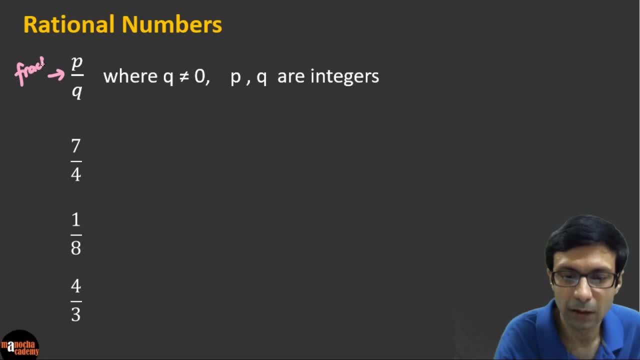 So can you see this fraction here? So rational numbers can be expressed as a fraction, as a p by q form Right. And note that the denominator q should not be equal to zero, Because why? You know that in maths, division by zero is not defined Right. 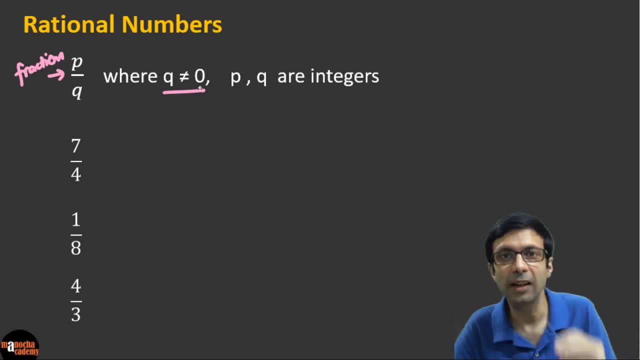 It's undefined. So rational numbers are basically fractions And we write it as the form p by q. And the important thing is, p and q are integers here. OK, So let's consider some simple examples here. So for example, can you see 7 by 4 here? 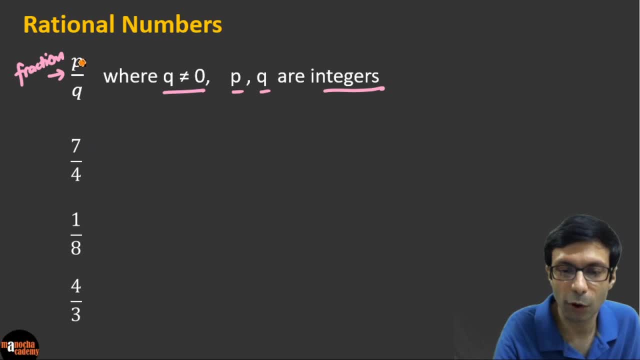 So if you look at this example- 7 by 4, can you see it's of the form p by q, Right? So if I write here p by q, can you see the form? So p is 7, q is 4.. 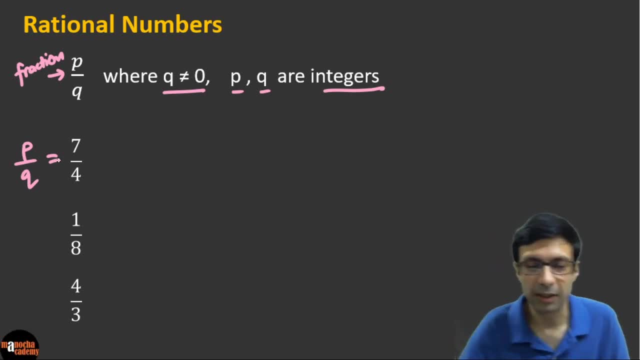 So 7 by 4 is a rational number. Similarly, if you look at the next example, 1 by 8.. Right, And the next example, 4 by 3.. So can you see that? So, guys, let's calculate these numbers. 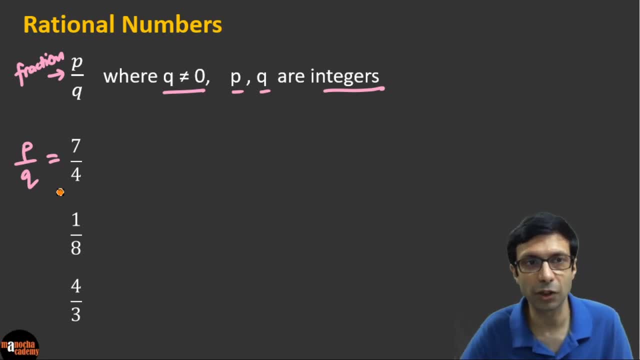 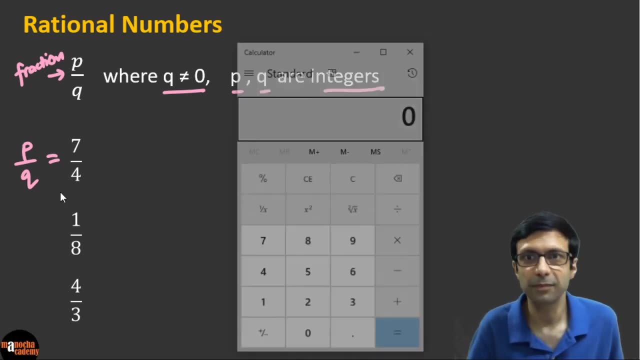 So 7 by 4,, 1 by 8, these are expressed as fractions And let's express them in the decimal form, Right? So I'm going to pull up the calculator here for you, Right? So actually you should practice division yourself. 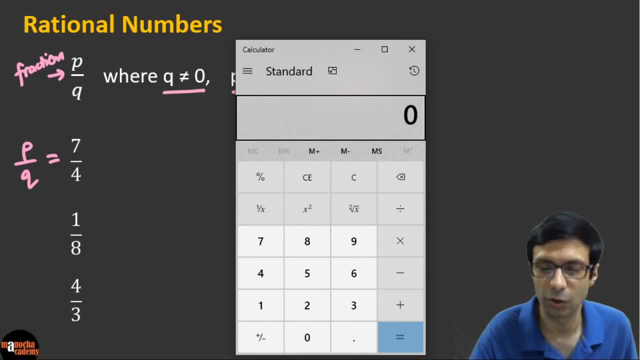 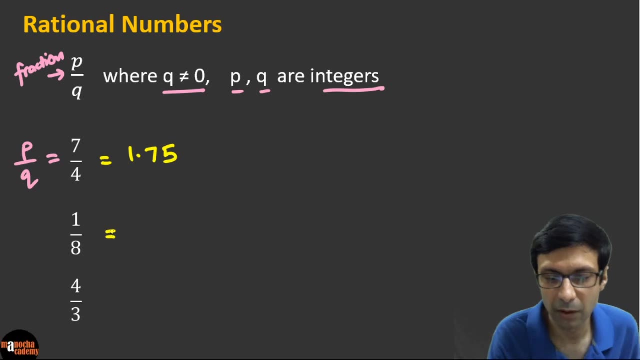 Let's take a look with the help of the calculator also out here. So 7 divided by 4.. Right, The first number. So that's 1.75.. Let's go ahead and write that down here. So this number is 1.75.. Let's check out the next number here. 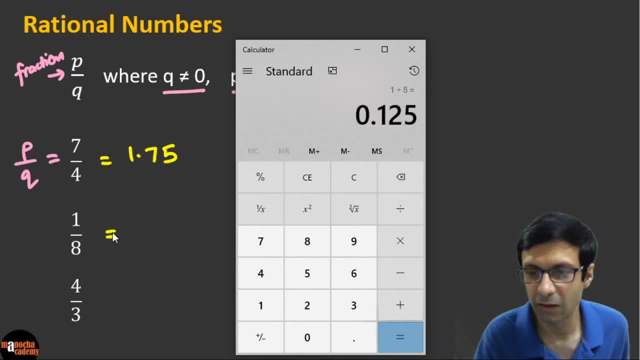 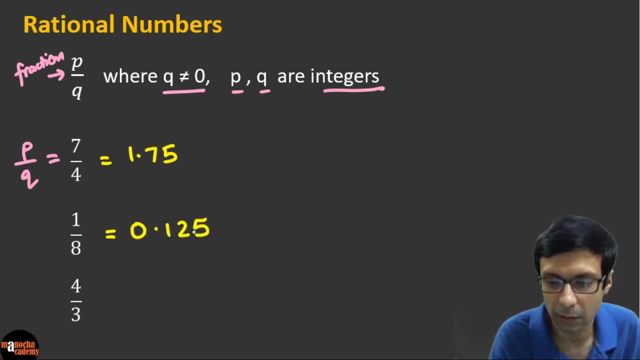 It's 1 by 8.. So 1 divided by 8.. Right, As you can see, it's 0.125.. Okay, And let's take a look at what is the last number here. So we have 4 by 3.. 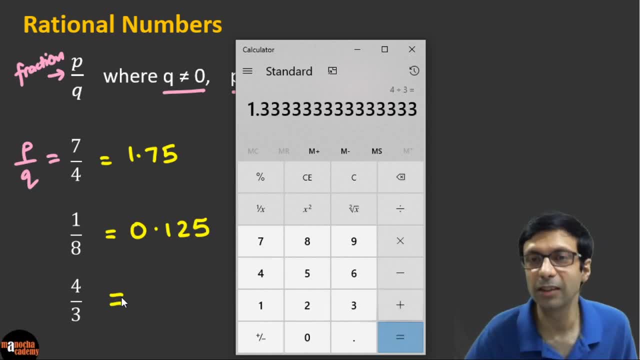 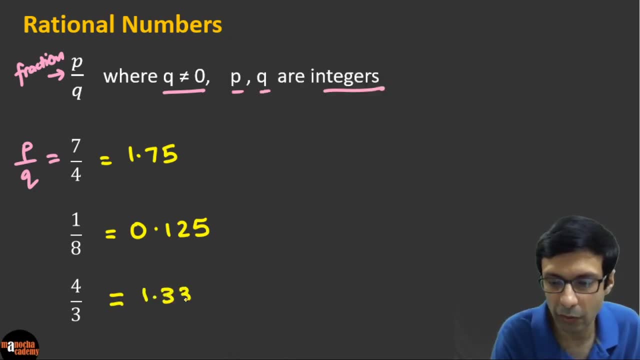 So 4 divided by 3.. Can you see in the calculator It's 1.333 and it just goes on. So I'm going to write that here. So 1.33333 and it just continues. Okay, So note what we've done here. We started with, we said rational. 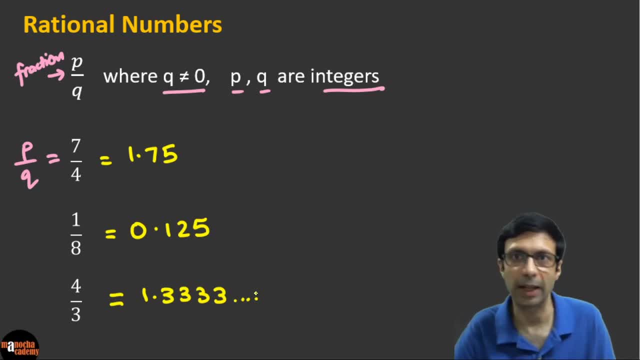 Numbers can be expressed as fractions of the form P by Q, Right, Where P and Q are integers, And here I have some examples for you. So we've expressed these fractions as decimals, Right? So now can you see. So what is the pattern that you noticed here, Right? 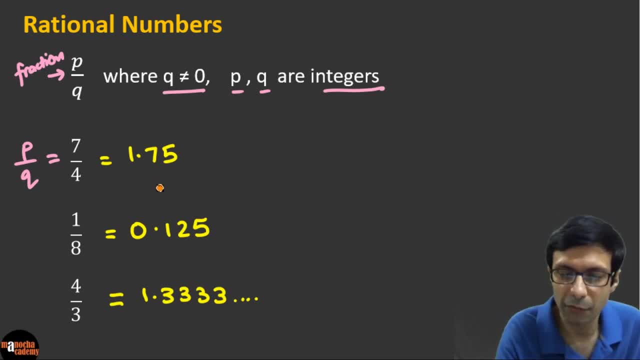 So can you see that in the first number, 1.75, and the second number, can you see that the decimal terminates, Right? So take a careful look here. So these are known as terminating decimals, terminating numbers, right, Because can you see that the decimal is terminating? 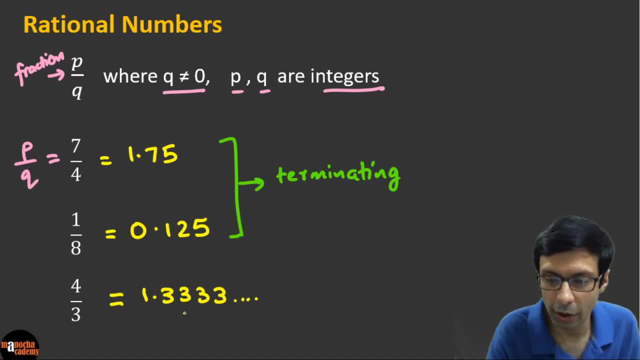 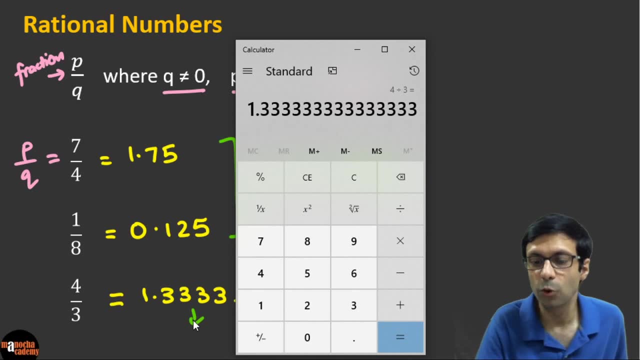 And if you look here, it's basically continuing on and on, So 1.33333,. it never stops right Because, as we saw here in the calculator, of course the calculator has a limit. You can't see the digits beyond the three. 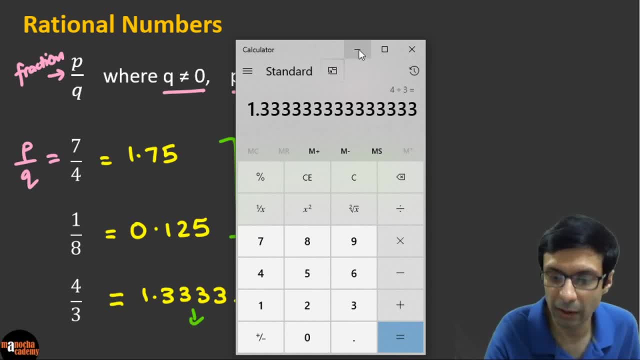 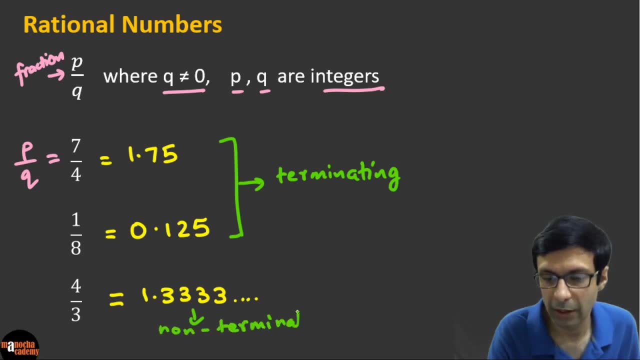 but can you see it's going on repeating 1.333?. So this is known as non-terminating And it's also called recurring. non-terminating and recurring, Right, Because can you see the number three is repeating here. Very good, 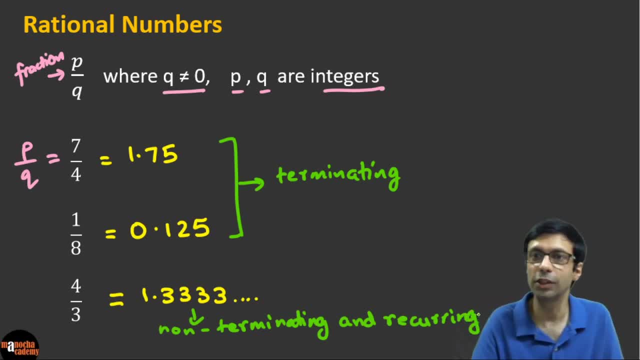 I see a lot of you have written non-terminating and repeating or non-terminating and recurring. Excellent, Right, And this is usually denoted in maths, as we say, because the digit three is repeating, So we do 1.3 and we put a bar on top right. 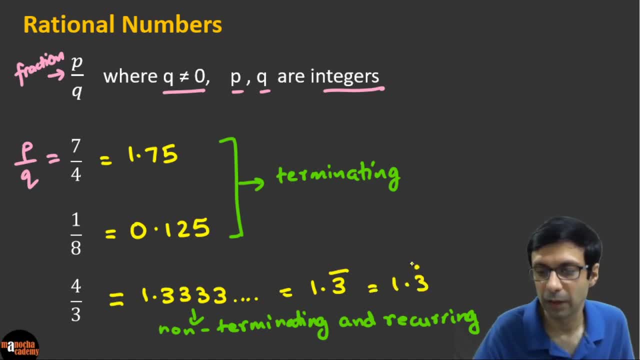 Or we can say 1.3 dot to represent that the decimal three is repeating: Excellent, Right. So look here, guys, this is a very important so you really need to understand these terms and concepts. So in rational numbers, you can express it as terminating. 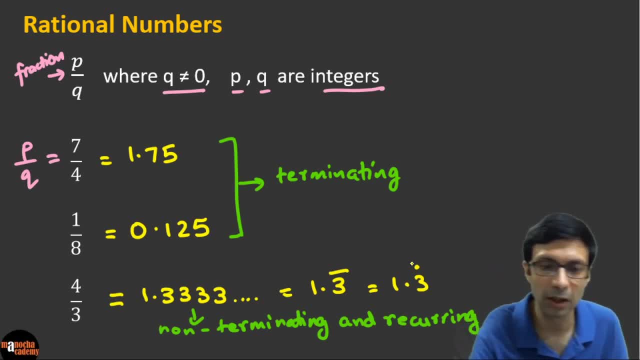 You can have in rational numbers, we can have terminating decimal numbers. So can you see these? So these are terminating decimals, or you can remove it as terminating, You can abnormalize it, have non-terminating and recurring, clear, excellent. so now let me ask you a couple. 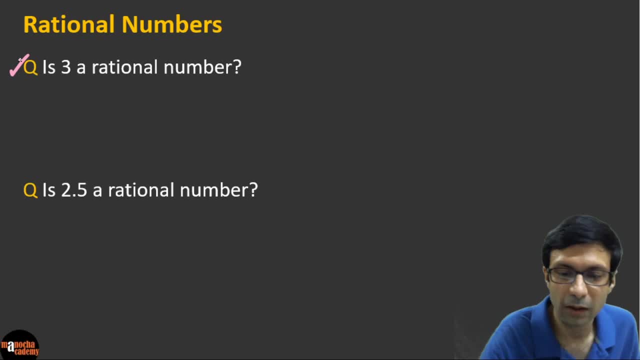 of questions, so why don't you go ahead and try the first question here: is 3 a rational number, yes or no? what do you think? so the first question is: is 3 a rational number? so I see Ayush says yes, Gautam Devnath says yes. right, yes, no. 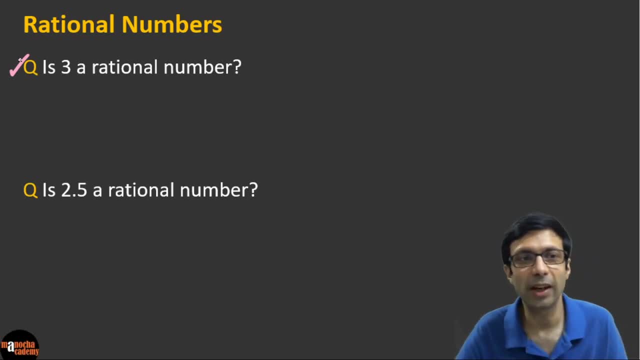 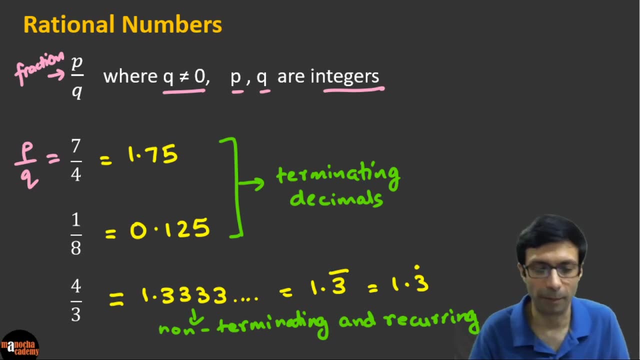 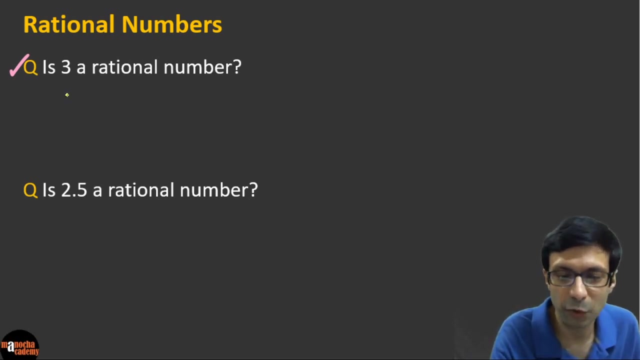 there are some no's here. so what do you think? is 3 a rational number or not? so what was our definition of a rational number? it should be of the P by Q form, okay, so why is 3 a rational number? so good, I see some of you have written the 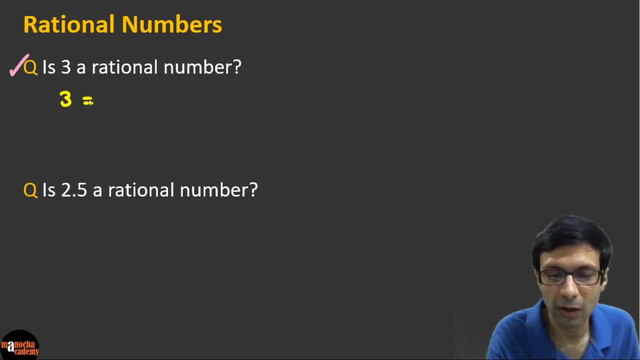 explanation also. so if you take the number 3, we can write it as 3 by 1, right? so here the denominator is 1 and can guys, can you see that? 3 is a rational number? so if you take the number 3, we can write it as 3 by 1, right? so here the denominator is 1 and can guys, can you see that? 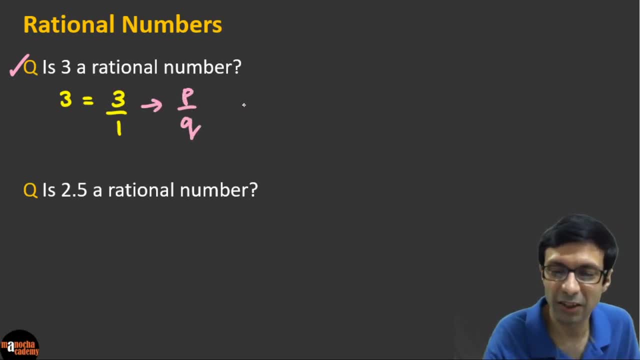 P by Q form here, so 3 by 1. so the answer is yes, 3 is a rational number, excellent, very good. now can you try the next question: is 2.5 a rational number or not? what do you think? so let's try the second question here, guys. so I see. 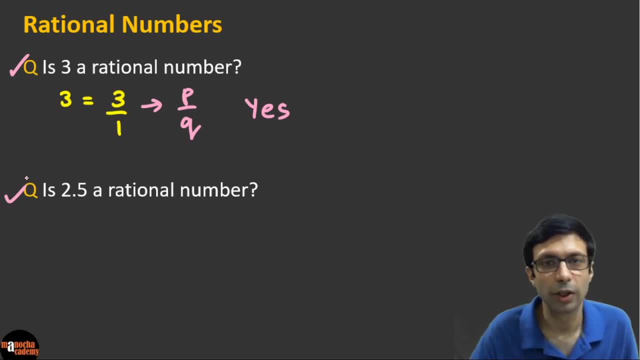 yes, yes, no, right. so is 2.5 a rational number? so again, we'll do the same thing. so if you take 2.5, it's in a decimal form and rational numbers are P by Q, right, because you can always convert decimal to fraction, fraction to decimal, right. so for these, 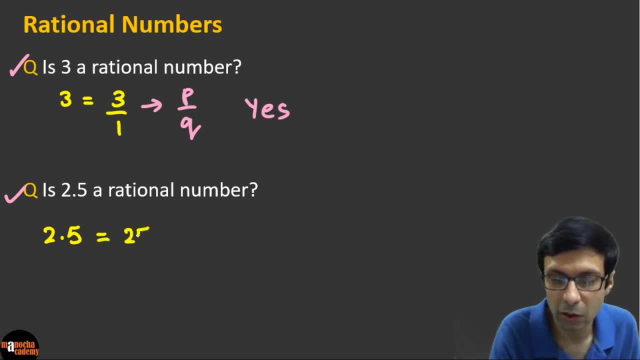 simple things. so for 2.5, what can be right? so we want to try to get it to a fractional form. is that possible or not? so we've got 2.5. so 2.5 is going to be 25 by 10, and you can simplify that, right. so it's going to be 5 by 2, right, okay so? 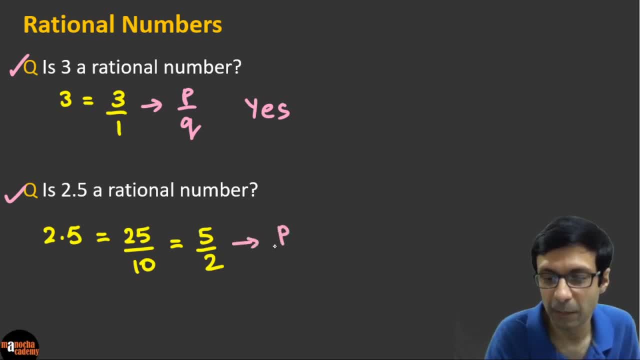 it's going to be 5 by 2 and can you see, it's clearly the P by Q form 5 by 2. so this is definitely a rational number. so the answer here also is going to be yes, excellent, so 25 by 10. 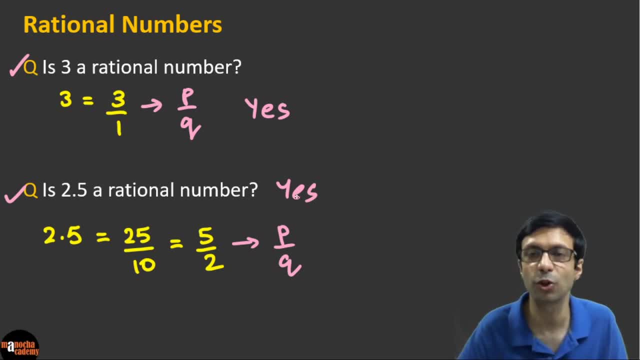 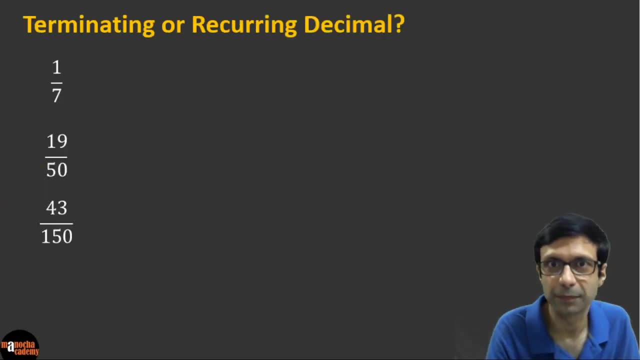 or you can. I'm seeing a lot of people are writing 25 by 10. that's also right, and you can further simplify it and cancel the common factor and it's going to be 5 by 2 super. so now let's take a look at these. so this is a very 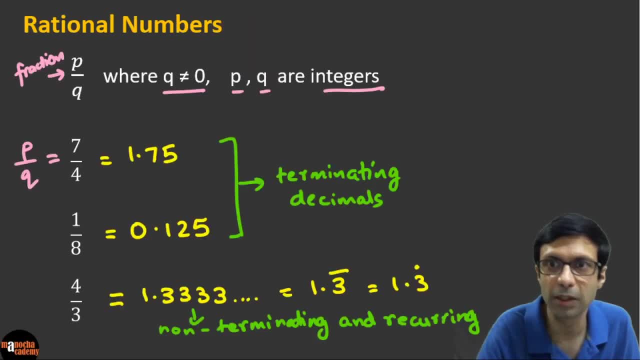 important and confusing thing, right? so we'll take a look at some more examples, because we talked about this concept of terminating means the decimal numbers stop after a point like this: can you see or non? terminating and recurring means they are going on endlessly. so rational numbers are of these two types, so let's 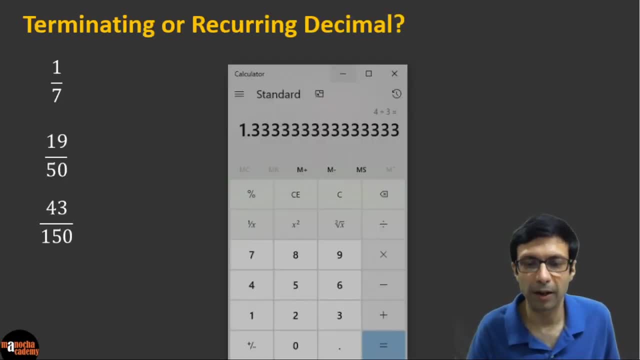 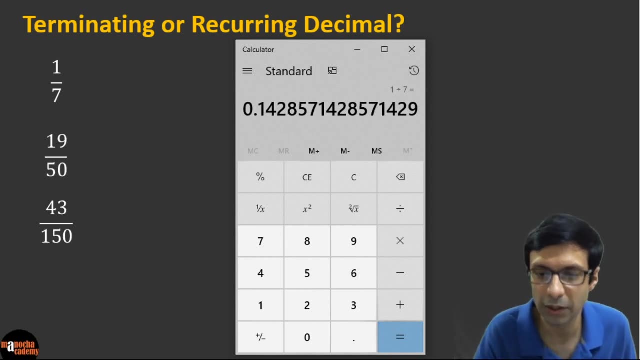 take a look at some more examples here. so again, I'm going to pull up our calculator and let's try this number 1 divided by 7, right? so you can calculate it yourself. for now we'll just use this. so what do we get here, right? 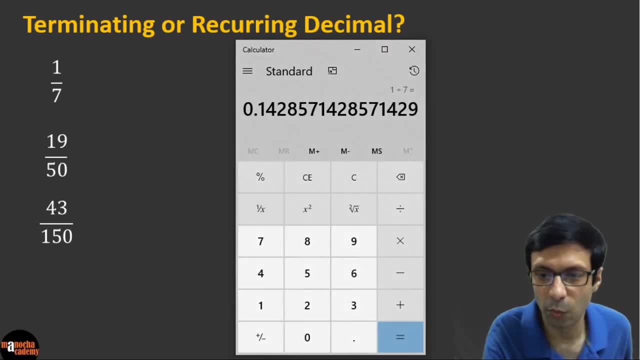 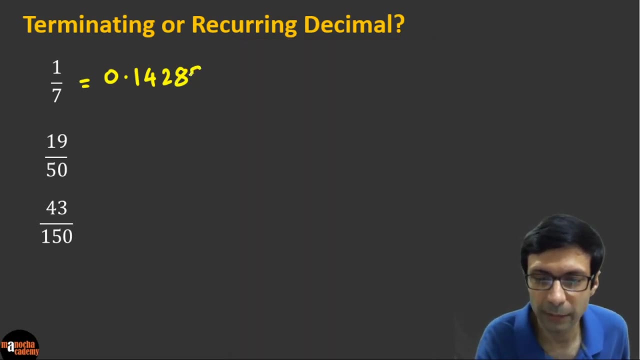 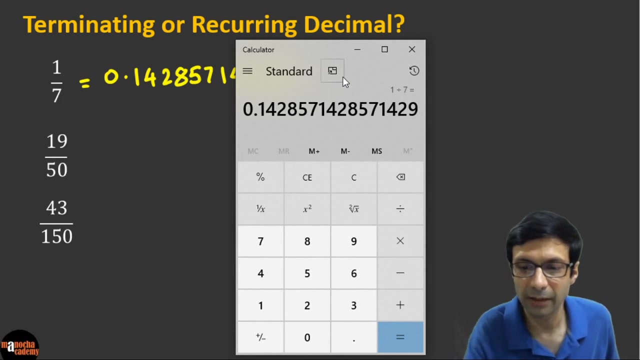 right. so can you see we are getting this thing 0.1428, so 285714 right and so on. so, guys, can you see that? so I'll just move this a bit to the side so you can compare this now. so, if you look at, 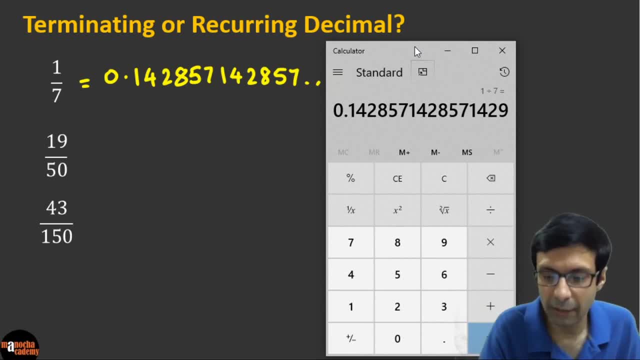 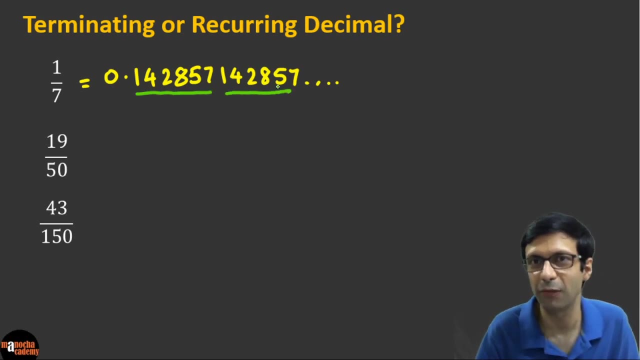 this number, 1 divided by 7, can you see? and what is the? so it is definitely it's not terminating, right? so 1 divided by 7, you can see it is continuing on and on. and can you see the repeating pattern? so what is the repeating pattern here? so 142857142857. 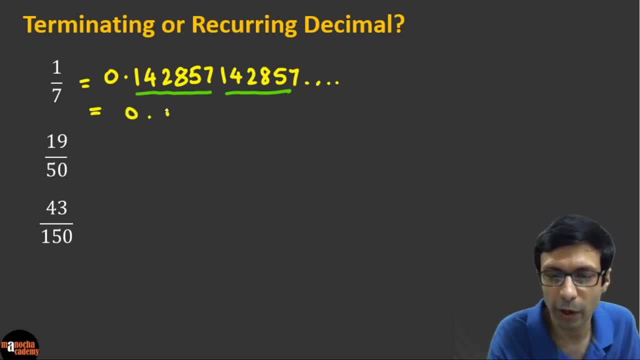 guys, can you see that? so we can write this of this form: 0.142857, where this part is repeating or recurring. so it's clearly a non-terminating number. so we can just see that and then we'll recurring decimal. So this one is clearly a non-terminating recurring. 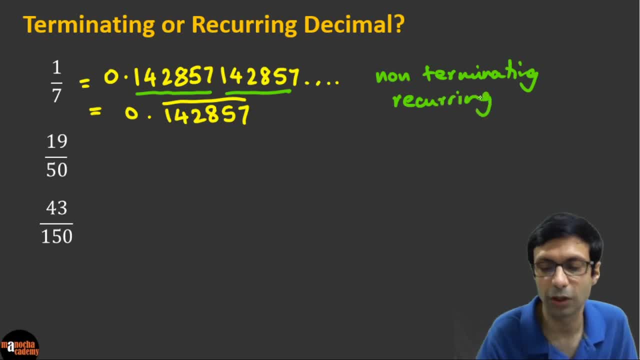 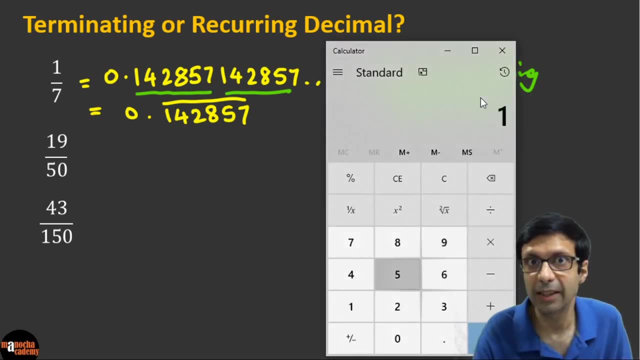 decimal. So it's a non-terminating recurring number. Now let's take a look at 19 by 50.. So again we want to decide: is it terminating or recurring? So again we'll divide and check right. So 19 by 50, sorry, not by 5.. 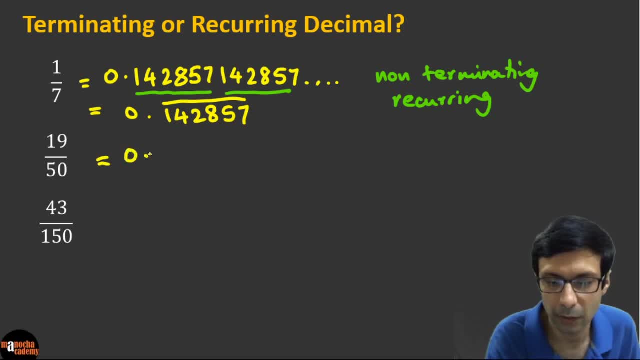 So 19 by 50 is 0.38.. Okay, and here can you see that it is a terminating decimal number. So here we are, doing all these divisions and finding it out. but I'm going to show you a simple trick where you actually don't have to do the 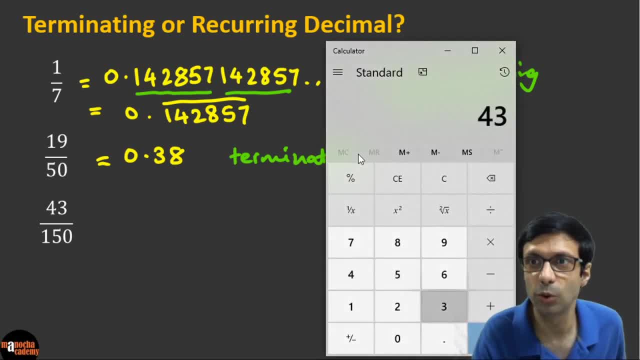 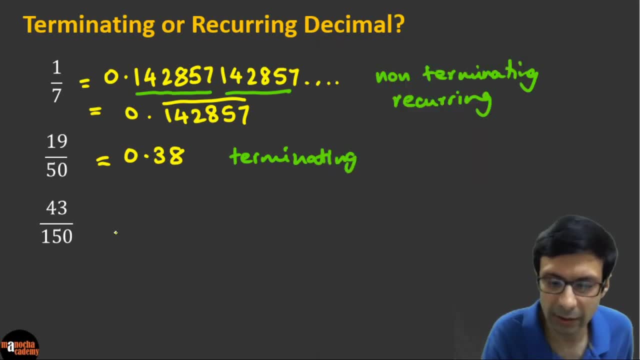 division. So I'm coming, we're going to come to that, and let's do the last number, 43. So let's call it 15 by 150 guys. So we are using the calculator here and can you see what do we get here, guys? So 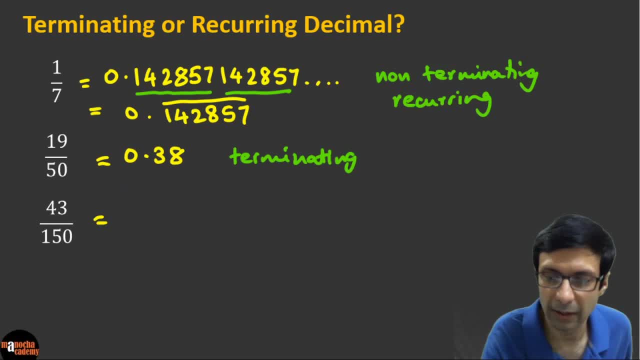 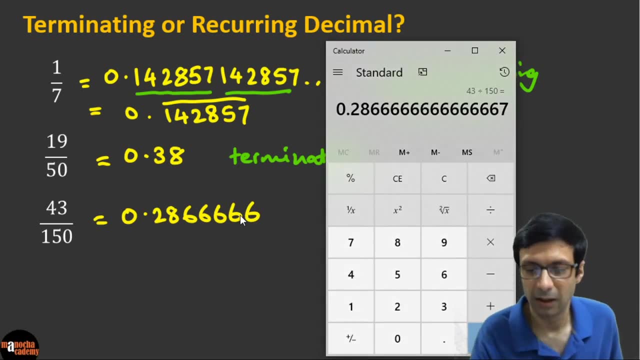 we're getting zero point two, eight, and then it continues, right. So zero point two, eight, six, six, and this thing goes on, right, Can you see that? and it's continuing. So we can express this of the form 0.28 colors and if you look at it now, it looks like that: 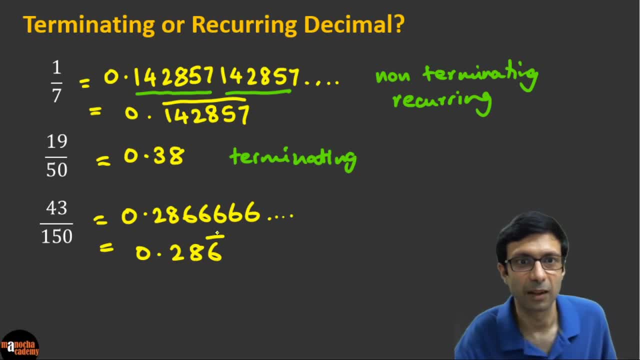 whether six is repeating. okay, And this is a. what is this going to be? it's basically, it's non-terminating, recurring. so non-terminating and recurring. and sometimes we simply say recurring because we know it's repeating, so it's not terminating, right? so 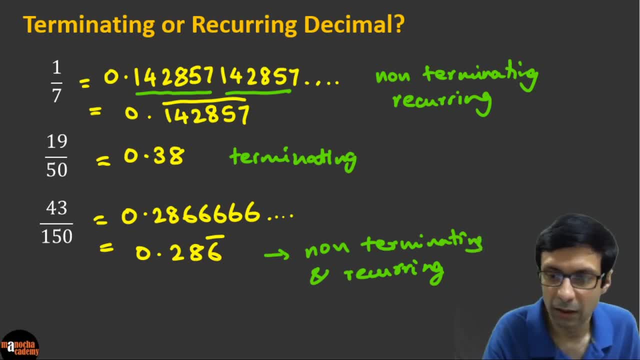 can you see here, guys, that this one, these two, were non-terminating and recurring numbers and this one was a terminating number, right? can you see that? so there's one important trick here. so one way is you can actually do the division. so in the exam and test you can't use a calculator. 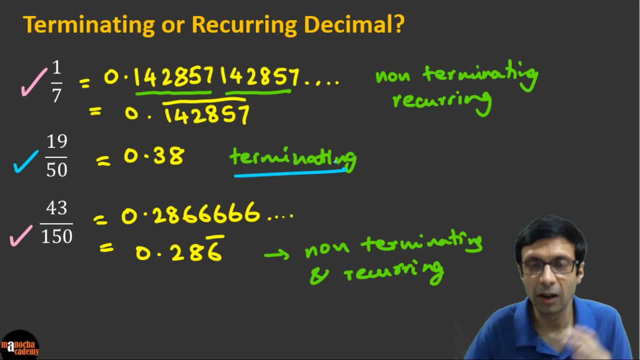 so you'll have to sit and divide. but there's a very nice trick where you can actually find it without calculating. so do you guys know what it's the trick? the trick is that you need to look at the denominator. okay, so we need to look at the. 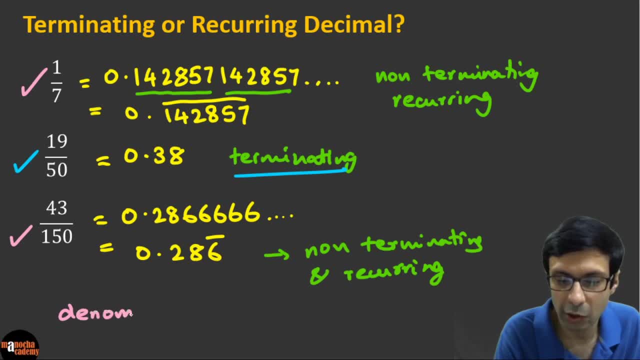 denominator of the fraction, and if the denominator has factors of two and five, only so, if it has factors of two and five only then, it is a terminating decimal number. so then it is terminating, then it's a terminating decimal number, otherwise it's going to be a recurring or a non-terminating. 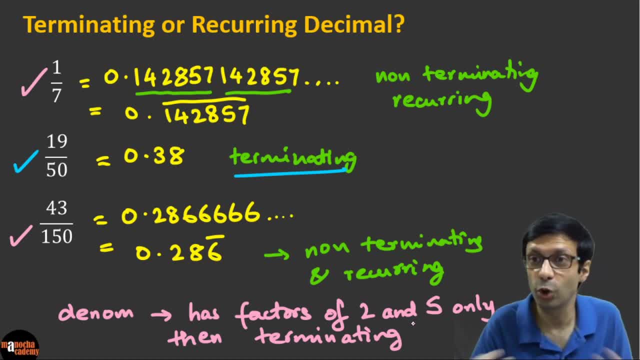 recurring decimal number clear. so see, guys, i've shown you the example of a calculator so you can practically try these also using your calculator, and understand it, to get a real feel of it. but now, if we apply this rule, let's see, then you don't have to calculate, okay? so what is the application of the rule here? 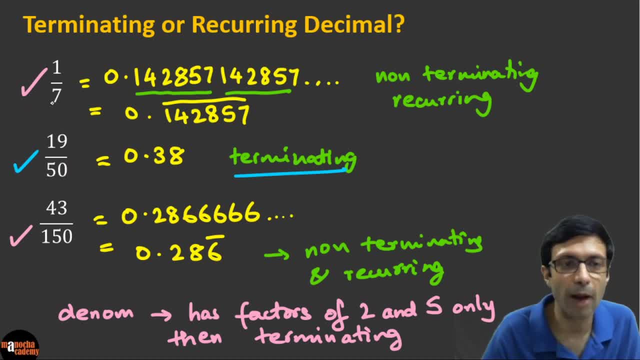 so if you look at the first first fraction here, one by seven, can you see that seven does not have factors of two and five, right? so it's the number seven. so therefore it is not going to be terminating and that's what we found using the calculator. now, if you look at fifty fifty, we can break it down as two into five. 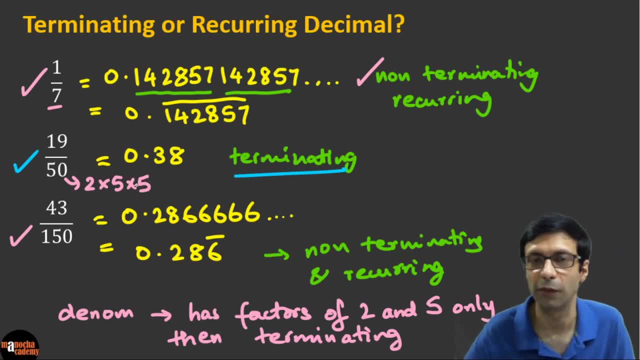 into five, right? so twenty five into two is fifty. so we've broken down and can you see that fifty has factors of two and five? only can you see that, guys? so therefore it's basically a terminating decimal number, as we marked here. can you see, we marked it as a terminating. 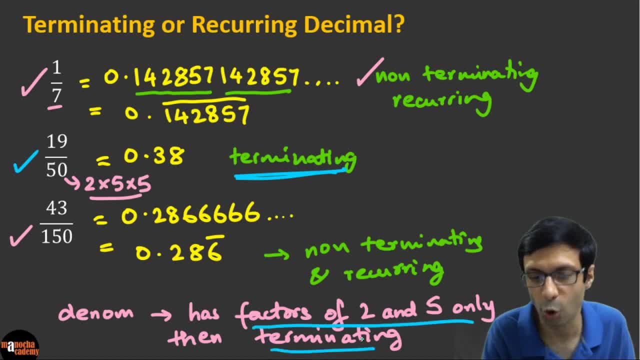 decimal number because it has factors of two and five only, and now, if you look at the last example, forty three by one fifty. so let's break that down. so what are going to be the factors here? so it's basically three into fifty, right, so it's going to be the 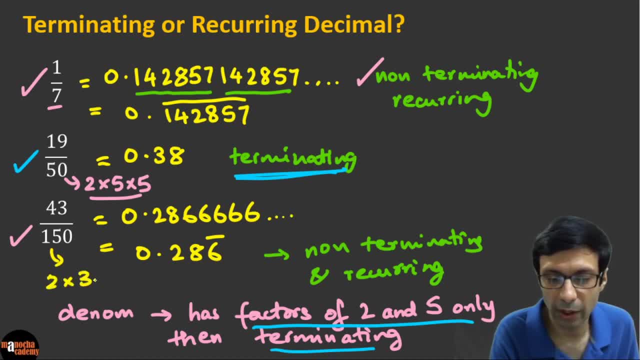 factors of this are going to be two into three, into five, into five, right, okay? and now can you see that we have factors of two and five, but it's not two and five only because we have the number three in there. so therefore it is non-terminating and 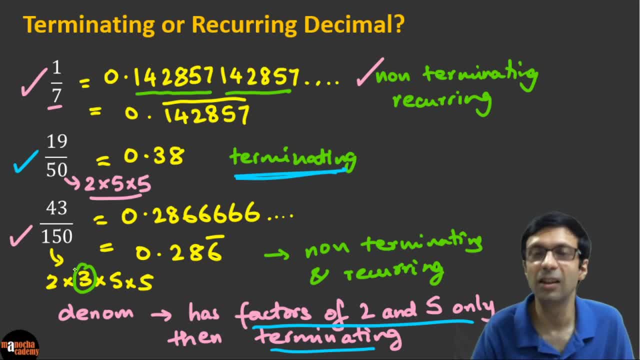 recurring. okay. so, guys, is this concept clear, that you actually don't have to do the division? you can use this simple rule that if the denominator has factors of two and five, only then you can surely say it's a terminating decimal number. otherwise it's a non terminating or recurring right. so here? 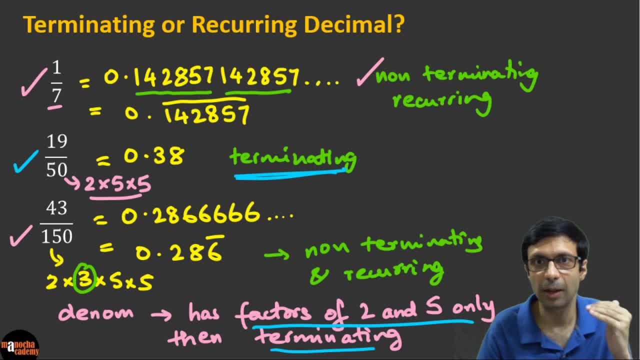 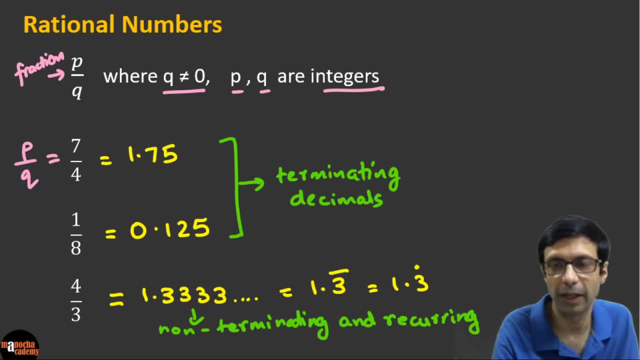 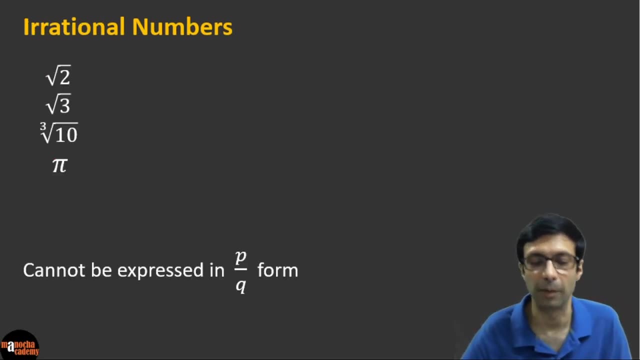 we talked about rational numbers. we discussed rational numbers of the form, which are of the form p by Q, and we divided them into terminating and non terminating or recurring terms. so now we, or recurring decimal numbers. Now let's go ahead and talk about another interesting set of numbers called irrational numbers. So what is the? 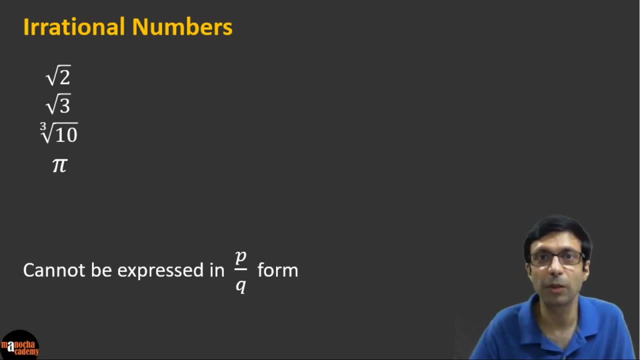 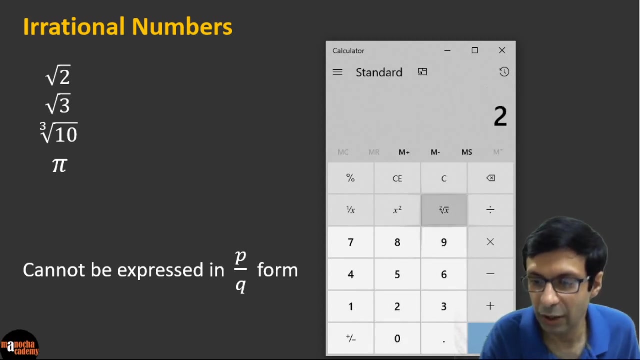 definition of irrational numbers. Irrational numbers are those numbers which are not rational. okay, So the numbers which are not rational, For example. so we have some examples here: root 2. So let's go ahead and take a root 2.. So if you do that in the calculator here, so can you see what do we have here? 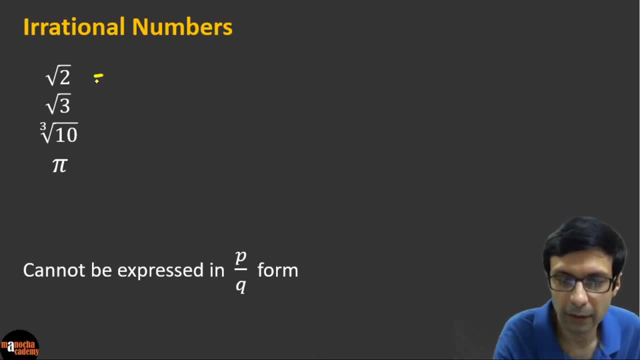 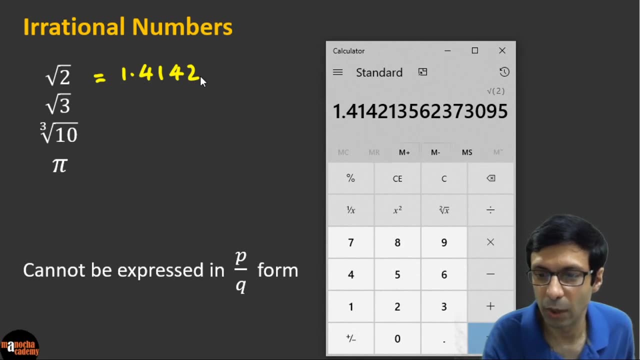 1.41.. So 1.4142, and let's write some more digits: 1356, right, Okay, guys. so can you see square root of 2? we have here similarly and it continues right, So there are more digits there. and then we have square root of 3.. So let's write: 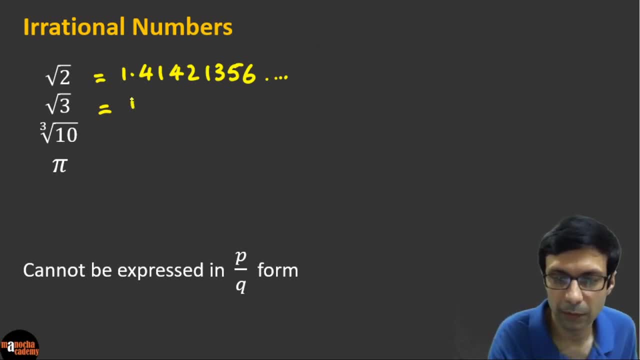 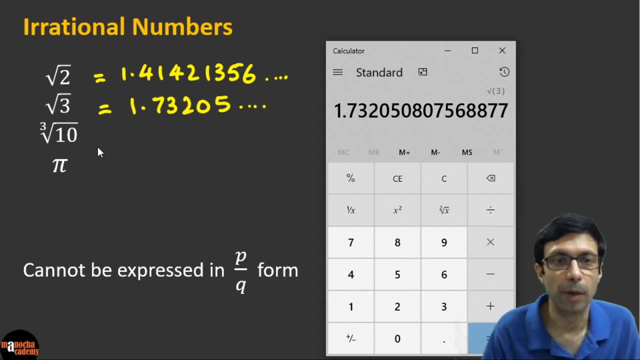 that down here, So 1.41.. 7,, 3,, 2,, 0,, 5, and it goes on. okay. Now, one important thing to note here is: these are also non-terminating, but are they recurring? No, Excellent, I see a lot. 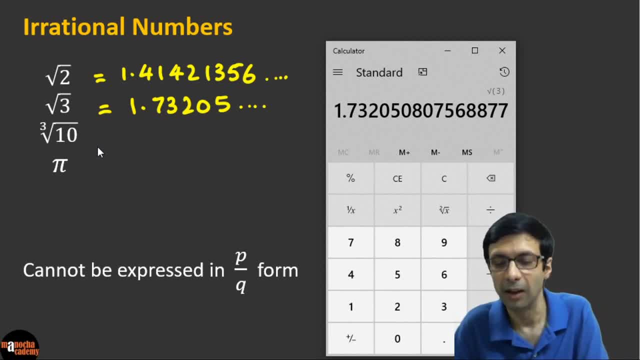 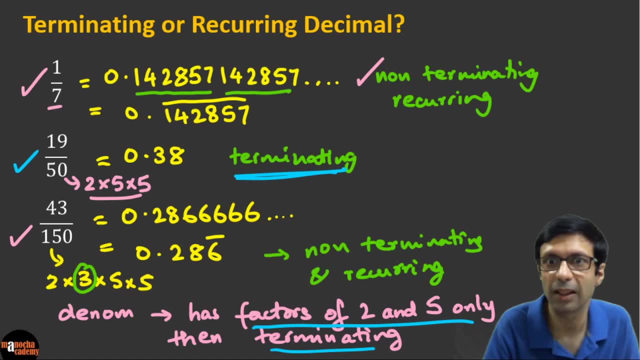 of you have written. they're non-terminating and non-recurring because you cannot find a repeating pattern here. Previously, remember we had found a repeating pattern in these numbers and that's how we had marked it with that bar and dot. but in these numbers, like square root of 2, square root. 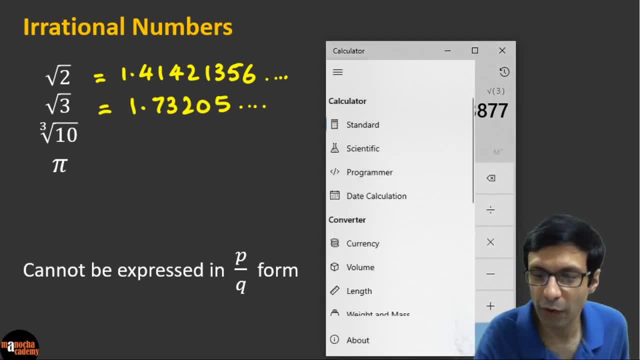 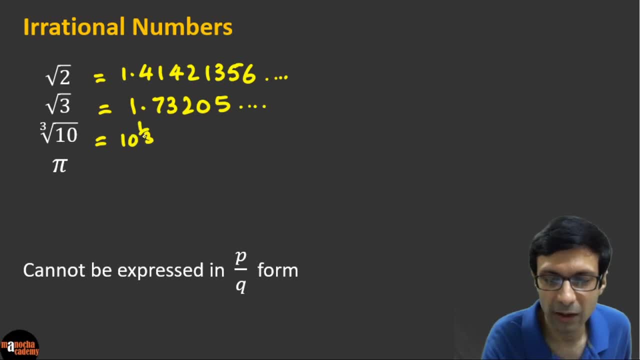 of 3 or, if you try, cube root of 10.. So, guys, do you know how to find cube root of 10?? So you're basically, cube root of 10 is 10 to the power 1 by 3, right So? 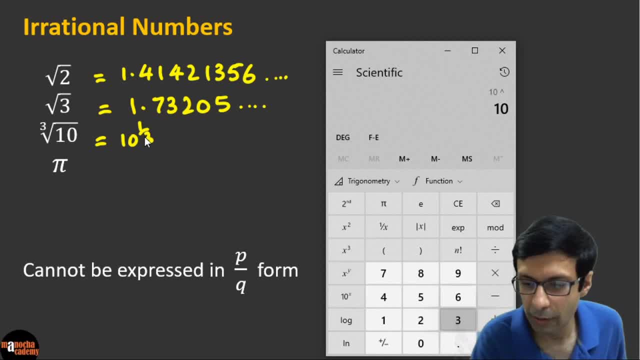 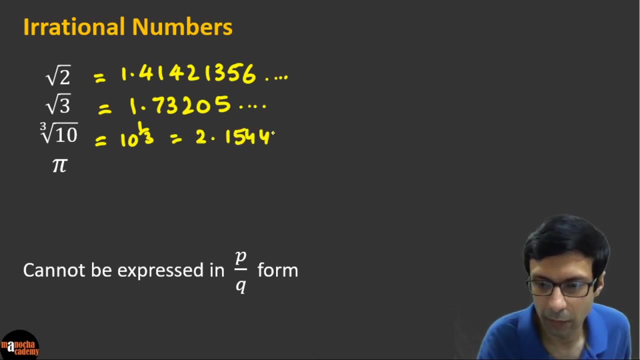 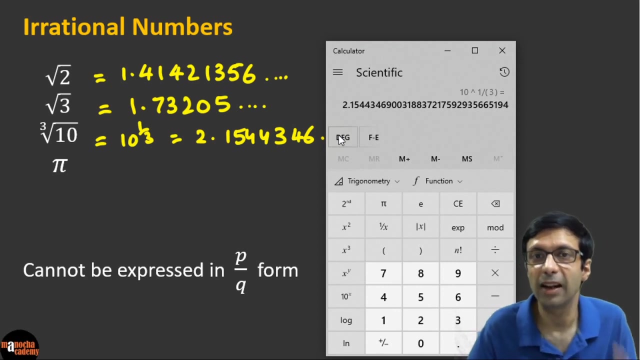 in a calculator, you're going to do 10 to the power, 1 by 3,, okay, and that's going to be the cube root of 10.. So it's 2.15443. we have here 3,, 4,, 6,, right, and it goes on, okay, So can you see that, the cube root of 10 again. 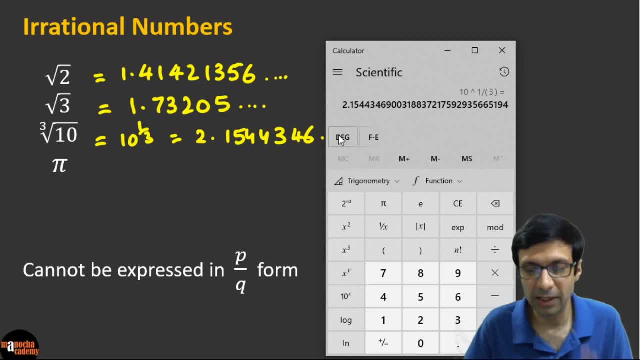 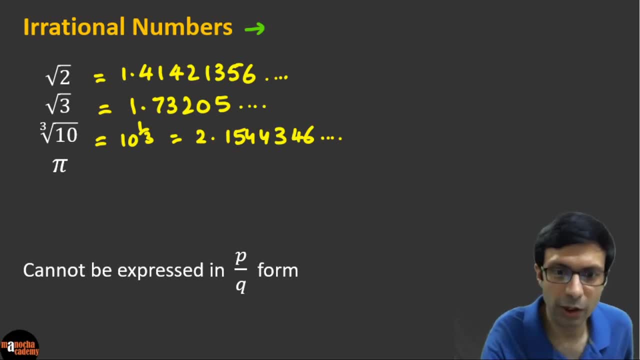 there is no repeating pattern here, okay. So these are basically so the irrational numbers, very important to note here. these are non-terminating, So they're non-terminating and non-recurring, okay. Non-recurring means they don't repeat, So please remember this important point. 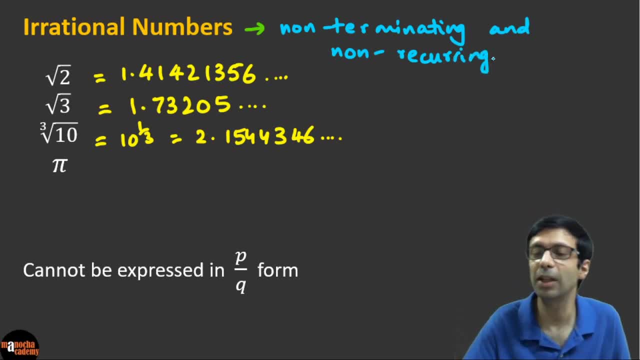 that irrational numbers. they have to be. non-terminating means they never end, So it can go on and on and on, and they're non-recurring, okay, And you may think that, oh, these calc, how do we know whether there's a repeating pattern? or 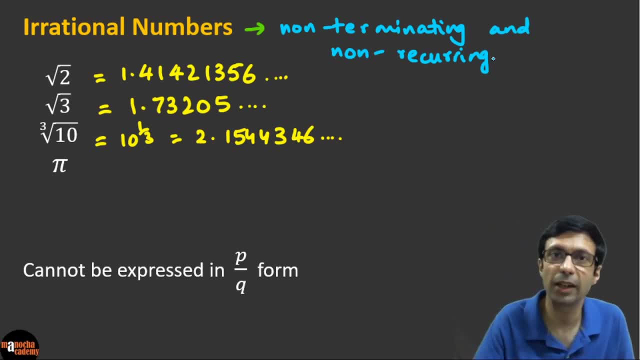 not Actually. they've used supercomputers and calculated these numbers till millions of decimal places and they have verified that these numbers root 2, root 3, cube, root of 10, pi, all these kind of numbers. there is no repeating pattern. 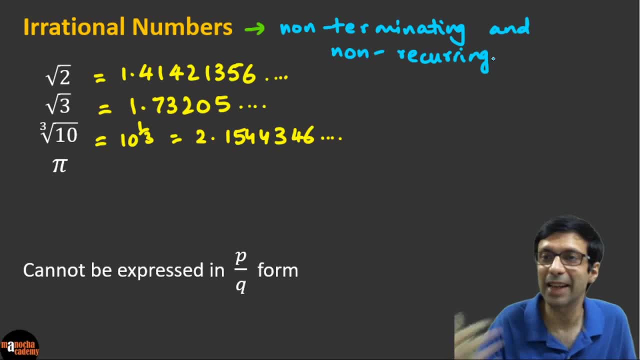 Okay, so the scientists have used computers and calculated it and checked that they are not finding any repeating pattern. so therefore they're definitely non-recurring and non-terminating. okay, And pi also. So please remember pi. normally you guys might be thinking we write pi as 22 by 7, right? So my question is: 22 by 7. 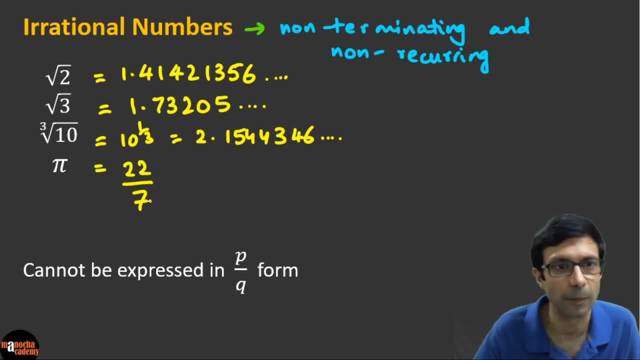 is that a round number? No, it is not. 22 by 7 is a number. So then why do we say pi is irrational? So do you guys know here, Right? So if we take pi as 22 by 7, is it a rational number? But normally we've studied in maths it's irrational number. 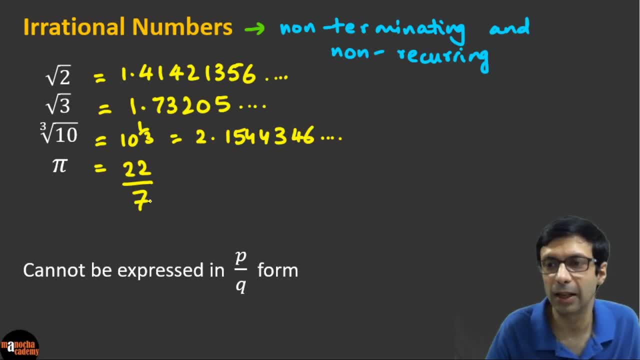 Okay. So what is the reason why 22 by 7 is not correct here? Because what's wrong about this is 22 by 7 is just an approximation. Okay, So that's only the approximate value of pi. So we are not going to consider that, because if you look at that then it looks like a p by q form, So it will be a rational number. So that's our approximate value. We won't take that. So you know that pi has the value and you can check in the calculator. 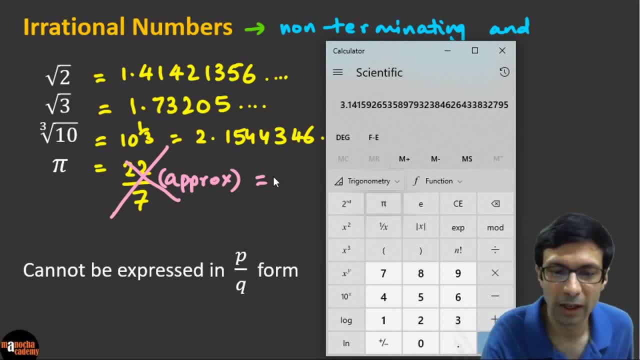 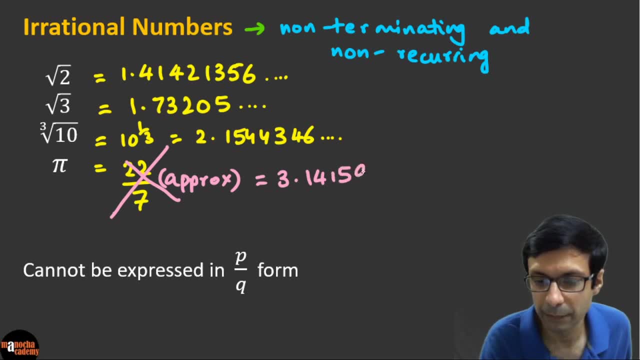 Also 3.14159,. you know it just goes on and on, So 3.14159.. Okay, So let me just erase this here and let's write pi again. So pi is basically so this is not the correct value. Pi is 3 point. It's only the approximate value. Right? And again, pi is non-terminating and non-recurring. 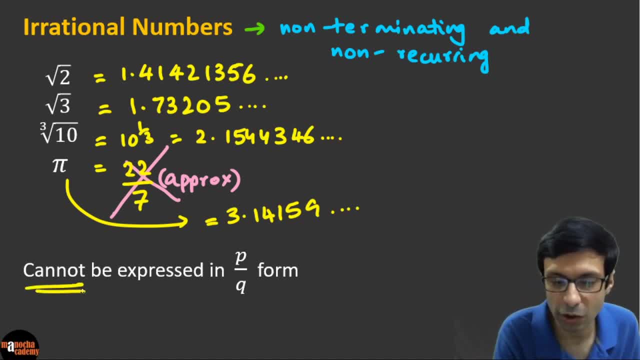 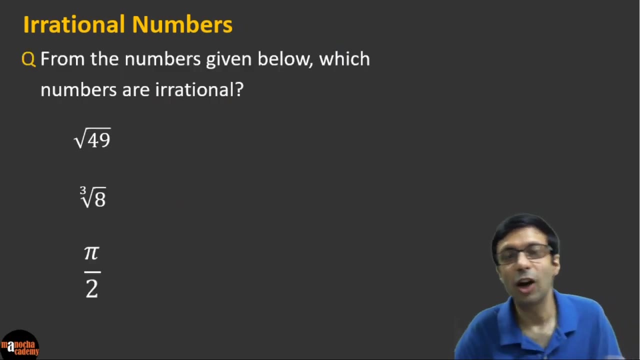 So the important thing, guys, the irrational number cannot, cannot be expressed in a p by q form. Okay. So please remember these important concepts, absorb them, Then you'll find this chapter really easy, because the definitions are very important. Excellent. So now I have some questions for you. So, from the numbers given below, can you tell me which numbers here are irrational? Okay, And one point: I forgot to mention these kind of numbers like root 2, root 3.. So these are known as: 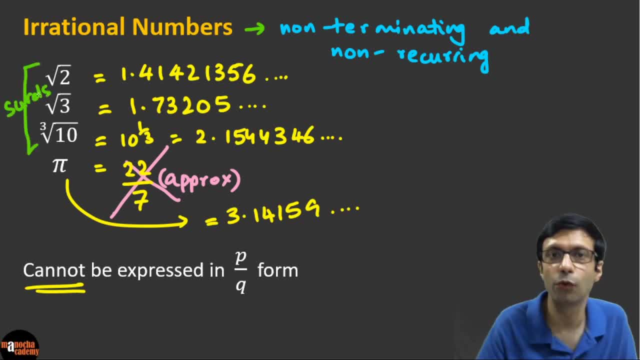 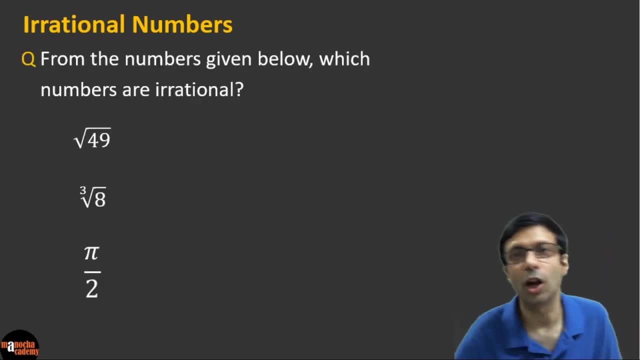 thirds: Okay, The square root form, the cube root form. So these forms are irrational numbers, right, They are good examples of irrational numbers. So now here's my question. So from the numbers given below, can you tell me which numbers are irrational? Okay, I see a lot of answers here, Good, So a lot of you are saying pi by 2 is the only irrational number here. Okay, Somebody saying cube root of 8, pi by 2.. Excellent. So from the numbers given below, can you tell me which numbers are irrational? Okay, I see a lot of answers here. Good, So a lot of you are saying pi by 2 is the only irrational number here. Okay, Somebody saying cube root of 8, pi by 2.. Excellent. So from the numbers given below, can you tell me which numbers are irrational? Okay, I see a lot of answers here, Good. So a lot of you are saying pi by 2 is the only irrational number here. Okay, Somebody saying cube root of 8, pi by 2.. Excellent. So from the 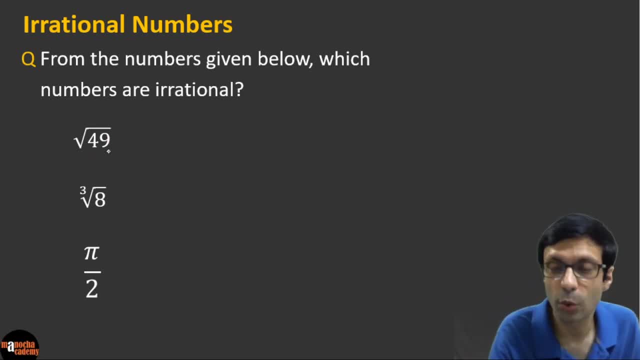 I think you guys got it right. so let's take a look, because square root of 49. so even though it's in a square root, it's in a third form, but you first need to check if it can be simplified. so square root of 49 is 7, so that's basically 7 or 7 by 1, right, and that's clearly a rational. 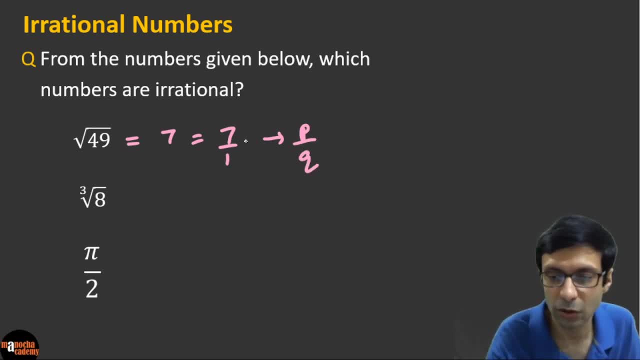 number because it's of the p by q form. so this is clearly a rational number. okay, now if you look at cube root of 8, what is cube root of 8? it's 2. so again 2 by 1. again it's of the p by q form, so it's. 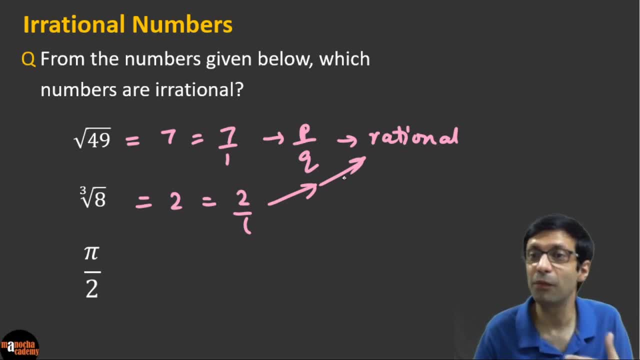 again a rational number, right? so remember to simplify. don't just assume you see a square root or cube root. okay, that's going to be irrational, don't make that assumption. but now, if you look at pi by 2 again, don't take pi as 22 by 7. that's only the approximate value. so as we 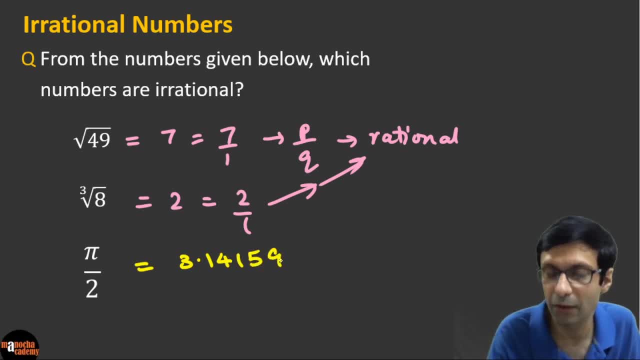 saw in the calculator, it's something like 3.14159 and there's like infinite digits, right. it just goes on and on. so if you divide that by 2, you'll still get a non-terminating, non-recurring number. so this is still going to. 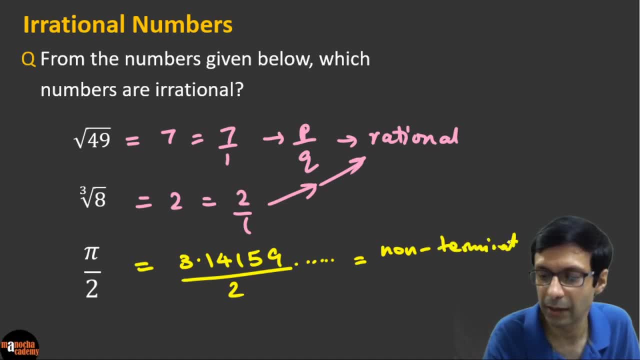 be non-terminating and non-recurring, so very important to understand these concepts. and non-recurring, and so definitely pi by 2 is basically an irrational number. so the only irrational number here from this list is pi by 2. excellent, i see a lot of you have got the correct. 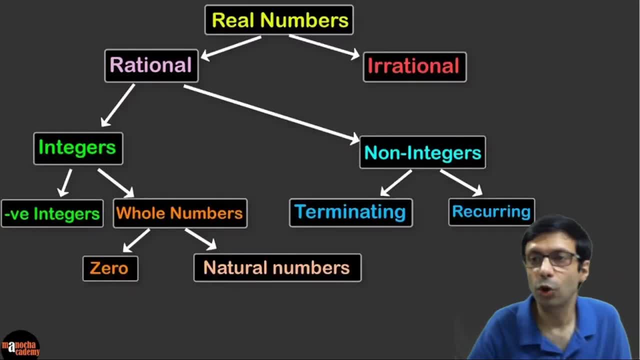 answer: superb, you, that's great. so we've talked about a lot of numbers, so let's visualize and organize this into this chart. and, guys, you can copy down this chart or you can take a screenshot of this or later copy down after the live session. so let's go from the top here and see: right. so 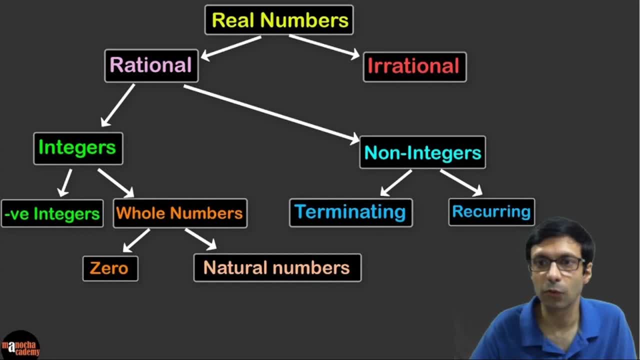 we talked about real numbers. right, we started with the concept of real numbers. real numbers are the numbers which can be represented on the number line. remember, we have done this number line here. so real numbers are numbers that can be represented on the number line and real numbers can be divided. 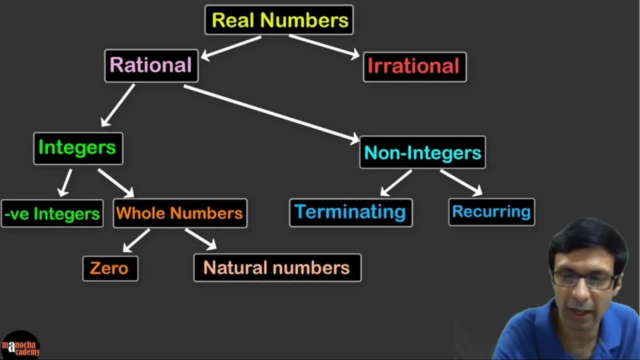 as into rational and irrational numbers. so, guys, can you see, real numbers can be divided as rational or irrational numbers. so we saw how to plot the integers, whole numbers and all, and even the fractions, and later we are going to take a look at how to plot the irrational numbers also, on the 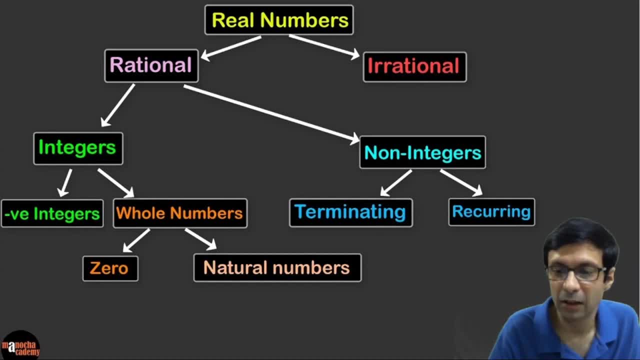 number line. so that's coming up, so let's see here. so what are the? and rational numbers can be divided into integers and non integers. right, and under integers you can have negative integers or whole numbers, which can be divided as zero or into natural numbers. so let's take some examples. so, for example, here, zero is here, and if you have numbers, 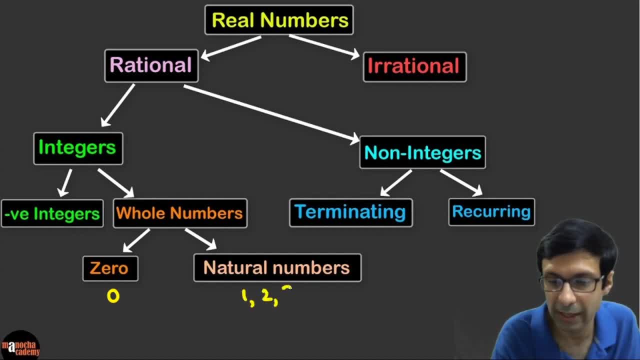 like one, two, three. the natural numbers will fall in this category, and together they're known as whole numbers. okay, and then you have negative integers like minus one, minus two, minus three, and so this entire set- okay, not just the negative integers, the entire set of negative integers. and 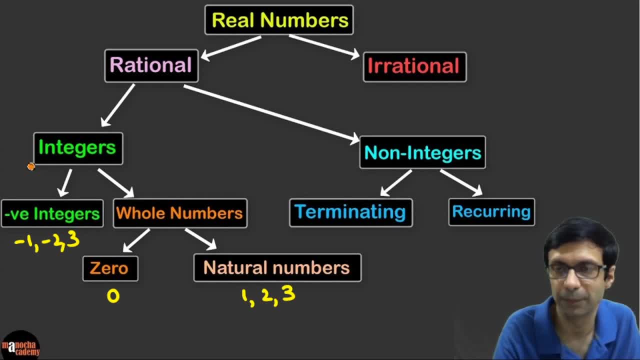 the whole numbers is together known as integers, right, so very good. and now, if you take a look, then there are the non-integers, so the things which are not integers, right, like decimals and fractions. so as we discuss, the decimals can be terminating. okay, so you can have terminating. 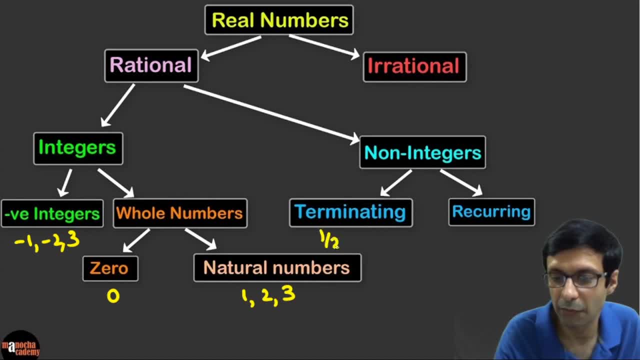 decimals, like. a simple example, is half right, half is going to be 0.5, so it's a terminating decimal. or you can have non non-terminating, which means recurring decimals, right. so something like 1 by 3, because you know it's 0.333, it goes on, so 0.3 bar, right. so can you see that non-integers can be divided into. 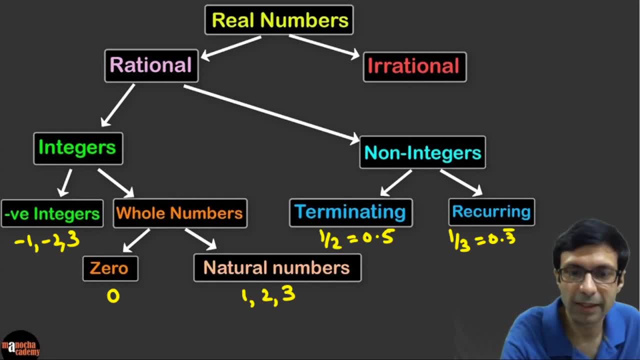 terminating and recurring. so this means that these are terminating and non-terminating, or basically recurring. so please make this important concept here, right and now. if you look up, so then if you go back to the real numbers, so these are all of these together, so all the integers and non-integers are together known as rational numbers, right? 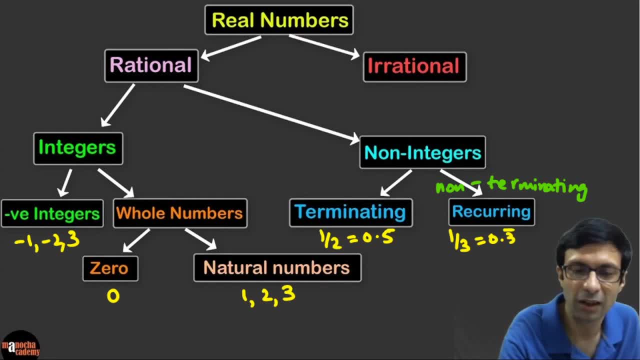 and those numbers which are not rational are irrational and we saw the examples. for example, you have root 2, square root of 3, square root of 2. you have numbers like pi right cube root of 10, as we saw. so these are all irrational numbers and the important thing to remember that the 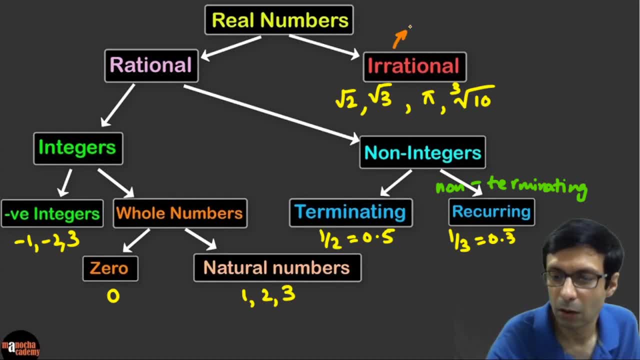 irrational numbers. they are basically non-terminating, non-terminating, non-terminating, non-terminating, non-terminating, non-terminating and they are non-recurring. okay, so i see some of you are writing imaginary numbers. so, for classes 7 to 10, imaginary numbers. 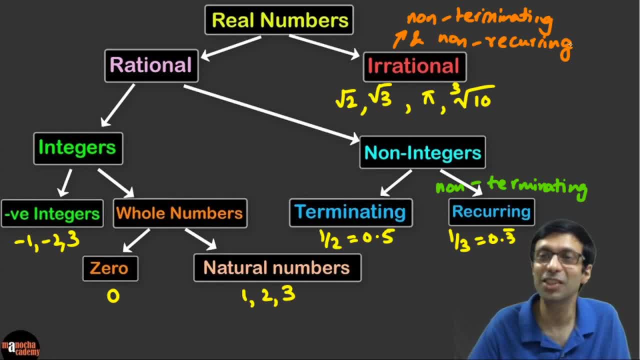 are not in the syllabus. so what is an imaginary number? a number which is not real. okay, so those numbers which are not real are called imaginary numbers, but we are. i have not put it in this chart because that's not in your syllabus, but note this very key definition because people get confused. 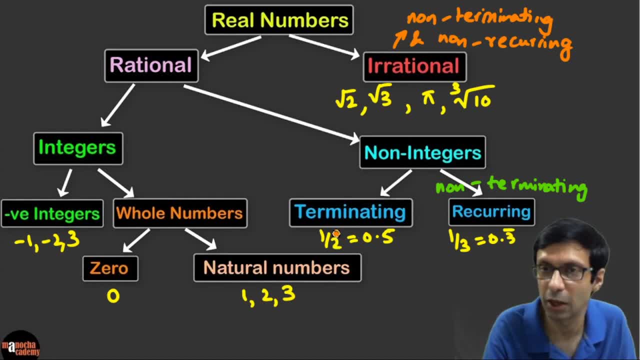 that we are not in the syllabus. so we are not in the syllabus, so we are not in the syllabus. but note this very key definition because people get confused: integers, the non integers, can be either terminating- that is simple. decimals are not terminating right- and recurring, so it's non-terminating. 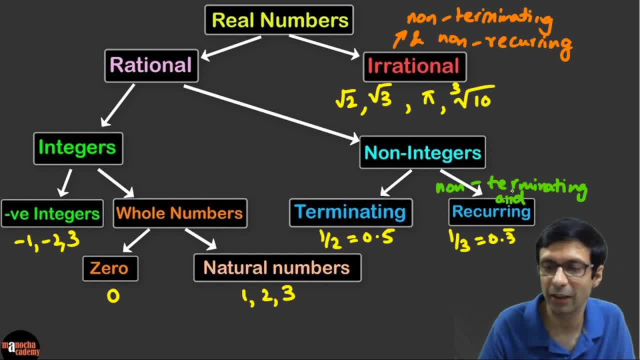 and recurring, which means the pattern repeats, or sometimes, which is one of three, or, and the irrational numbers are only, and they can only be non-terminating and they have to be non-recurring, so they should be DR, all right, can visualize this and you'll find it real easy, and i highly recommend you to draw this chart also. 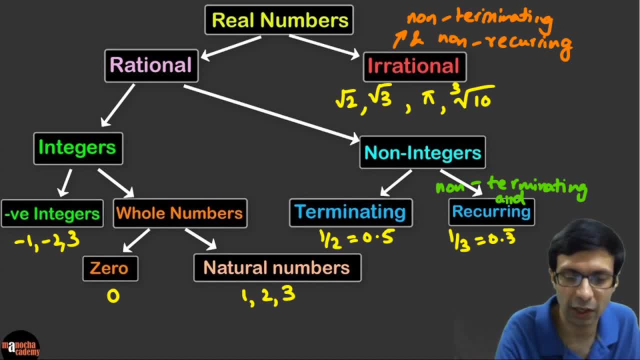 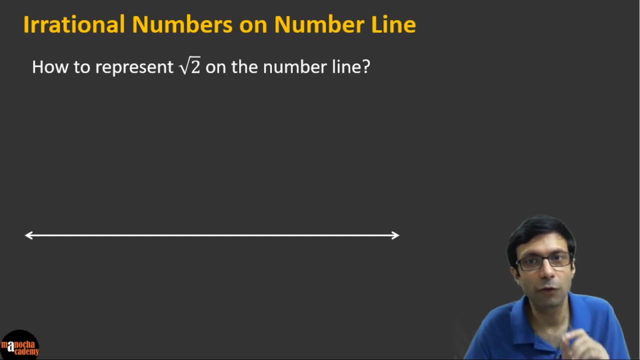 on paper. right then you'll completely absorb this classification. because you know so many terms, it can get confusing. all right, excellent. so now let's come to this interesting topic, that: how do you represent irrational numbers on the number line? so, for example, if i have to plot, 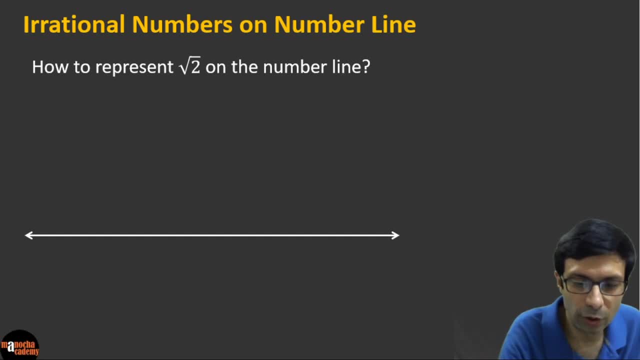 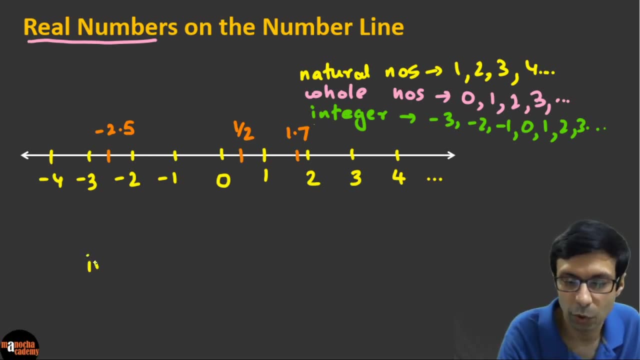 root 2. okay, so we looked at this number line here, right, remember, guys? so suppose we want to plot the irrational number, which is also a real number, right? so if you have an irrational number like square root of 2, how do i plot it accurately on the number line? okay, 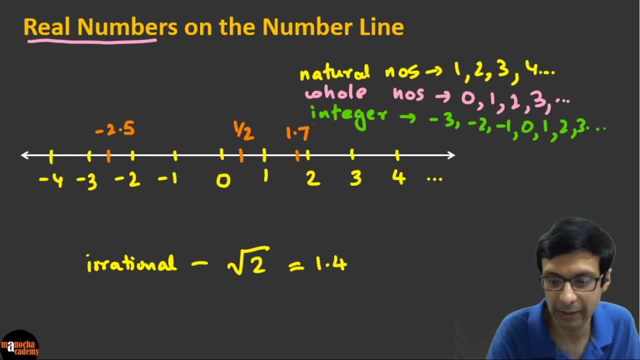 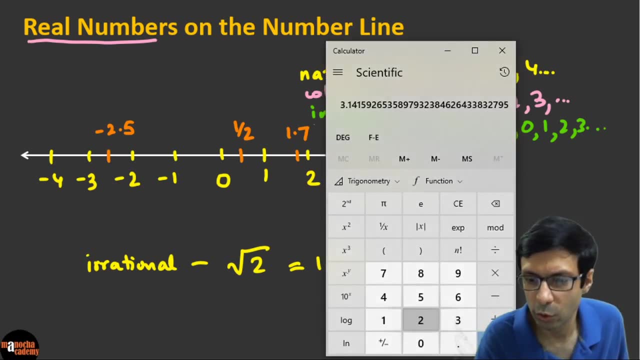 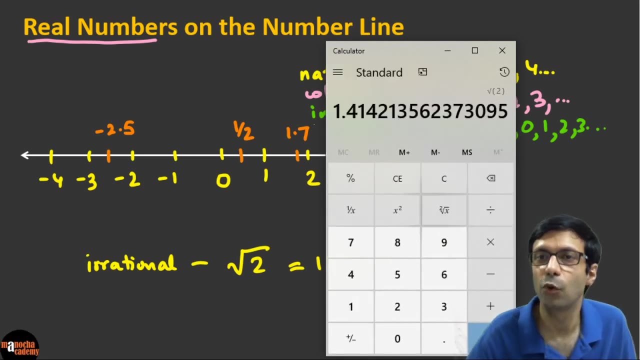 we know that root 2 is 1.41 right, 414 right. so if you look at the calculator right, so square root of 2 is going to be one point four, one, four, two right and so on. but this is endless right. so how do we accurately? 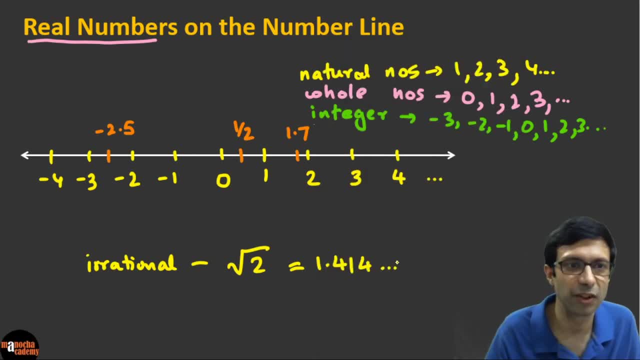 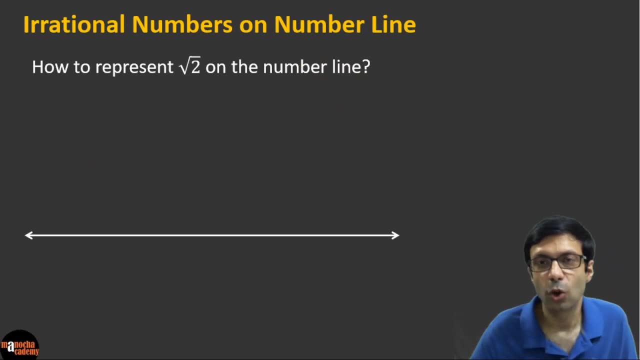 plot this guy. so that's the interesting question, right? so let's understand that. so i'm going to go down here and let's take a look at this. so how do we plot root 2? so very good. some of you are saying pythagoras excellent. so yes, we need to. 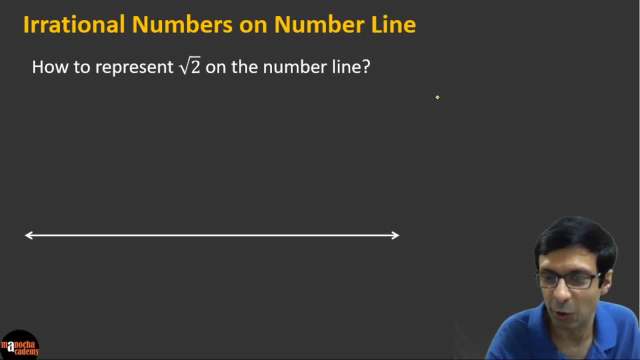 to use Pythagoras theorem. So let us understand how. okay. So let us say, you take, so you consider, a triangle like this right? So how can we represent root 2?? So if you take a right angle, 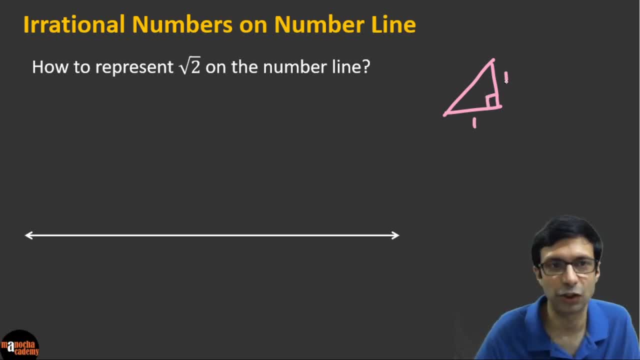 triangle where these sides are one unit each. okay, Excellent, lot of you are saying Pythagoras theorem. So if these sides are 1 and 1, if we apply Pythagoras theorem, what is going to be the hypotenuse? So the hypotenuse is going to be square root of 1 square plus 1 square. 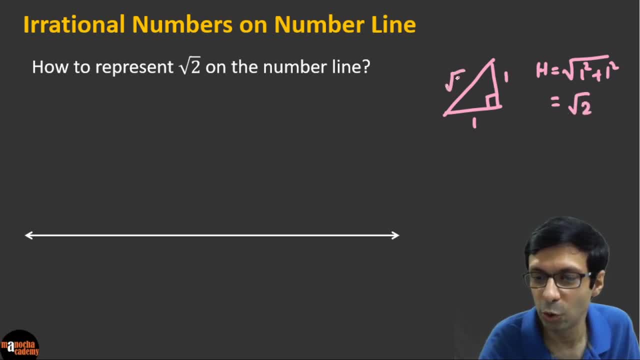 which is basically root 2, right, So root 2 is our hypotenuse. okay, So using this Pythagoras theorem, we are going to plot root 2 accurately, not roughly. okay, So we are going to plot root. 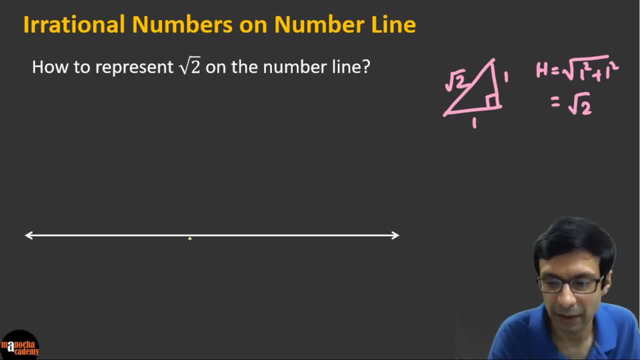 2 perfectly and accurately on this number line. okay, So let us take a look. So let us say our 0 is here. I am just going to draw it a bit to the left. And one important thing: do not mark 1 as 1 centimeter, because that distance is going to be. 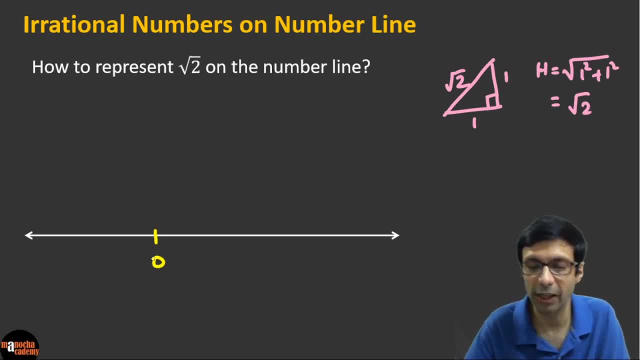 really small, So you can take 1 to be larger, like 1 inch or maybe 3 centimeters. So let us say your 1 is somewhere here, okay, And then your 2 would be somewhere here, and so on, okay. So I am just. 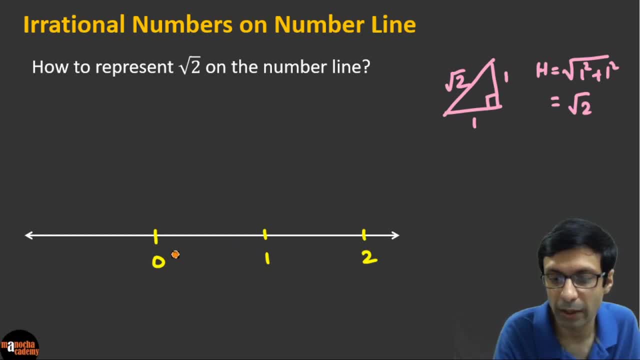 showing it roughly here, but you need to draw it accurately, with a scale where this distance is around 3 centimeters, so that it is easy for you to draw the diagram. So this is our side here, and it is basically represented by a square root of 1.. So let us take a look at this. So let us take a. 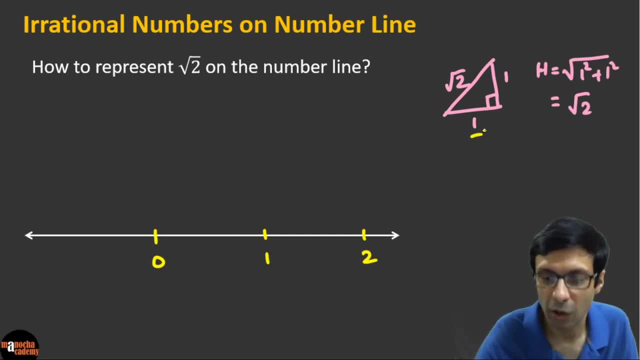 look at this side. So let us say this side is representing 1 unit, So it is representing this side. Now, what you do? so, using construction, you draw a perpendicular here. So we are going to draw a perpendicular, right? So let us say: this is our perpendicular, So I will draw it. 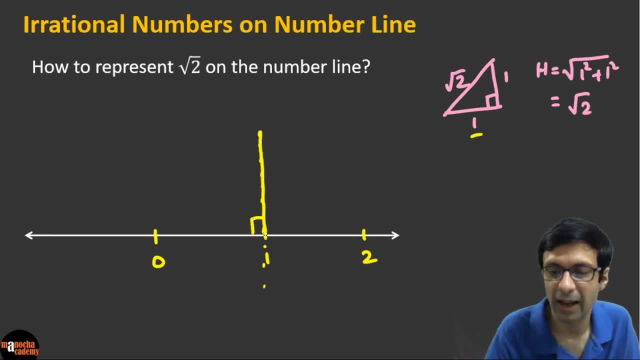 now with a solid line, and this is 90 degree, and let us say this thing: till here is 1 unit, okay, So this is 1 unit, right? And so let me just erase this. so this basically is one unit, so this is our one and this is our one, right? and now, if you join this, 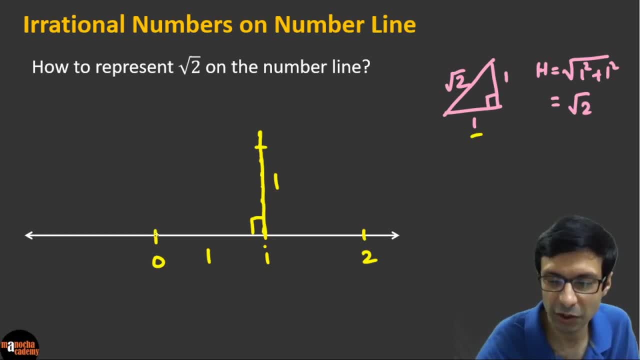 here. so this: you need to draw the perpendicular using construction. so i'm sure you know that and now, if you join this, so this length of this hypotenuse, as we discussed, is going to be root 2 clear. so, guys, we're using pythagoras theorem and representing root 2 here geometrically. 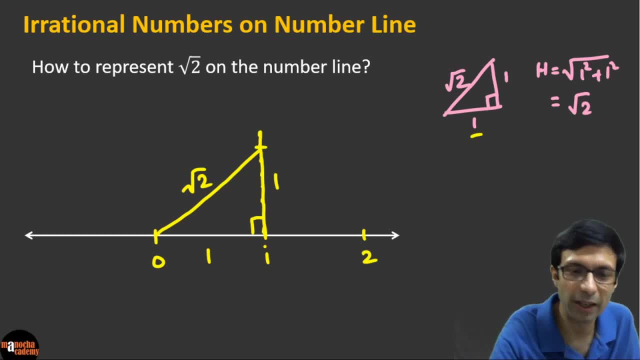 right. so using geometry, and now the important trick is: you put your compass at point o and where your compass is of this length, root 2, and you draw this arc. right. so you're going to draw this arc and you know it's going to fall close to 1.4, right, so it's going to. so if you complete, 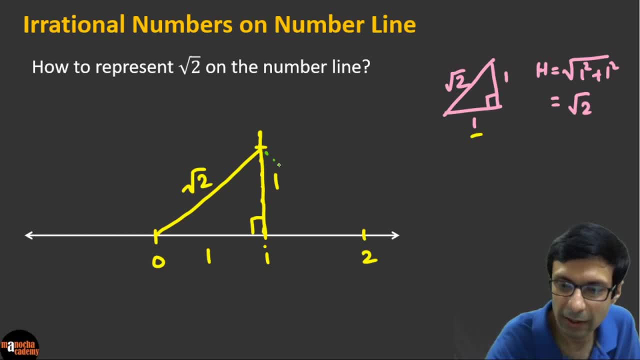 this arc here, right? so let's say, we draw the arc something like this, right, and so this point right here is going to be: so, this point where, uh, where you put the compass at this zero and draw this arc. can you guys see that? so, when you draw this arc, this is basically going to be your uh root 2 and we represented 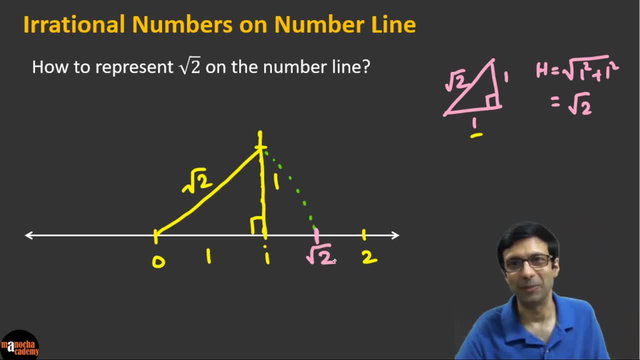 root 2 perfectly and accurately on the number line. excellent, right, so is that clear? so we basically use pythagoras theorem and found root 2 on the number line. now the question is: how do you plot? let's say we want to plot another number, let's say root 3. so, guys, how do we plot root 3 on the number line? so can you tell me that? 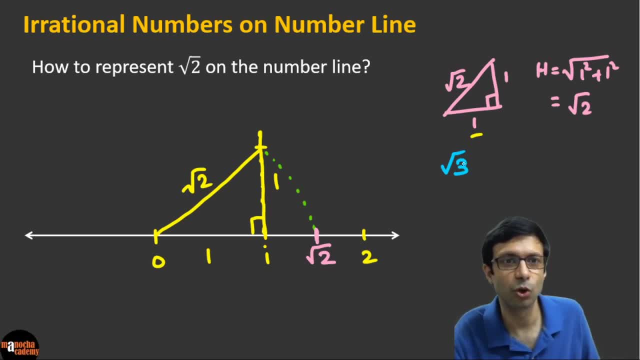 so we correctly represented, uh, root 2. so how do we plot root 3? so what do you guys think we need to do here? so yeah, somebody says, uh, arg, math says another triangle, right. so again, we need to apply pythagoras theorem, right, so in for this one. so what is going to be the sides of the triangle? 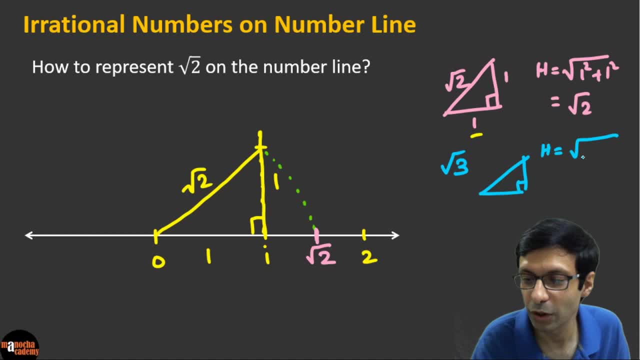 so for root 3, we're going to plot root 3 on the number line and we're going to plot root 3 on the number line. so root 3, you know, if you again apply the hypotenuse, so root 3 can be represented as: 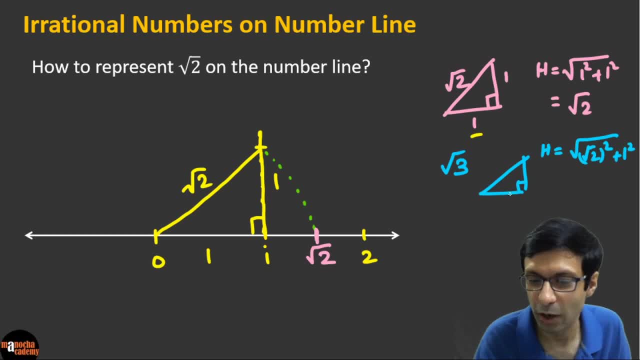 root 2 square plus 1 square, right. so one of the sides is going to be root 2 and the other side is going to be 1.. so, if you do the maths, so this is going to work out to be root 3, right? so can you. 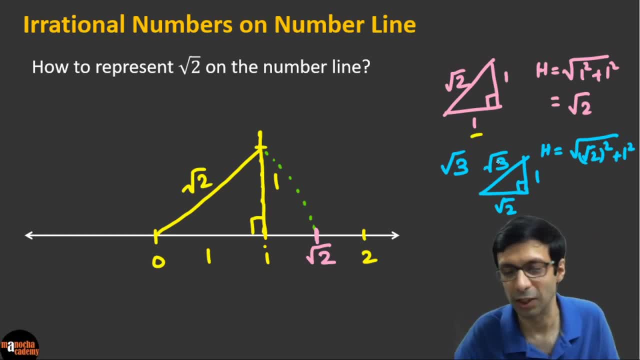 see that. so the hypotenuse is going to be root 2 square plus 1 square. okay, so now we're going to make use of this, since we've already found root 2 here. so what we're going to do is we're going to. 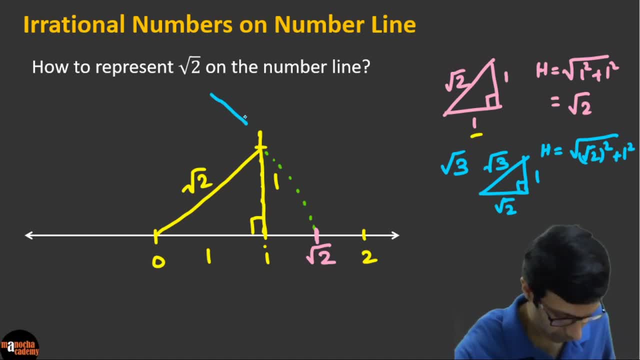 make a perpendicular here of 1 unit. so you can either do that on the number line or we'll do it here, right? so we're going to make a perpendicular here of length 1 unit. so this is 1 and this is perpendicular. it's perpendicular to this root 2 and let's complete this triangle now. 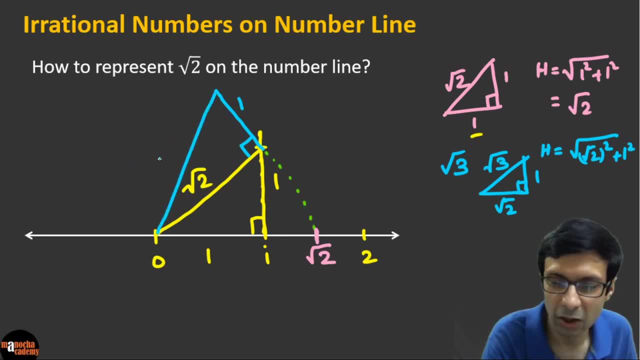 so, guys, can you see that? so what is this triangle going to be? this is root 3, right again, applying pythagoras theorem. very simple, so it's the square of root 2 plus 1 square, and again you take your compass and put it at o, and now, this time, you draw this arc. 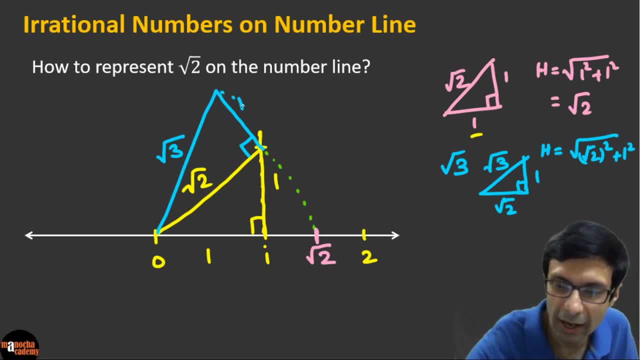 right. so if you draw this arc here, you know it's going to land up near 1.7, right? so the root 3 will land up somewhere here, and here we've got square root of 3.. so again, we plotted root 3 accurately on the number line. so is this point clear, guys? so what? 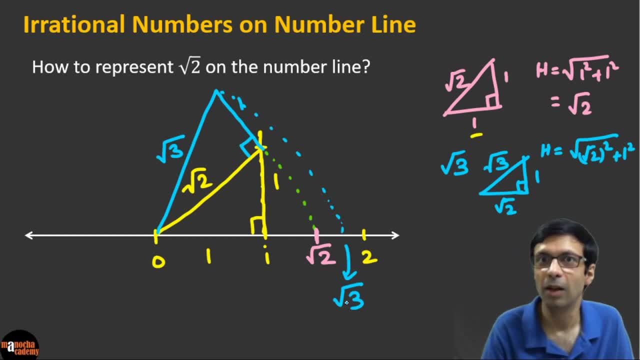 is the trick we are using here? we are using pythagoras theorem, because root 2, root 2, square root 3, these are non-terminating, non-recurring decimal numbers, right? you can't calculate them accurately, so we are using geometry to plot them on the number line. okay, and similarly another. 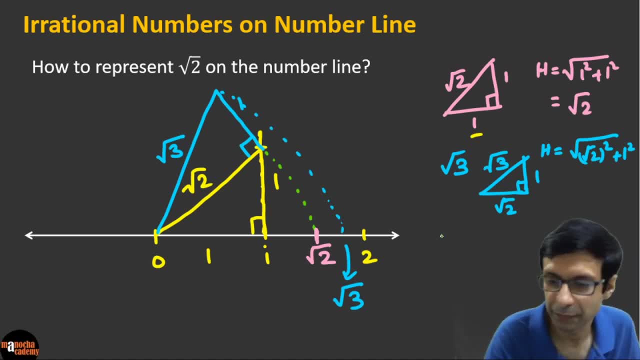 good example for you to know is root of 5, right? so how would you plot square root of 5 on the number line? okay, so how do you do that? so again, we can apply pythagoras theorem, right, so root 5 to be the Pythagoras theorem. So, for the hypotenuse, for root 5 is going to be square root of you know. 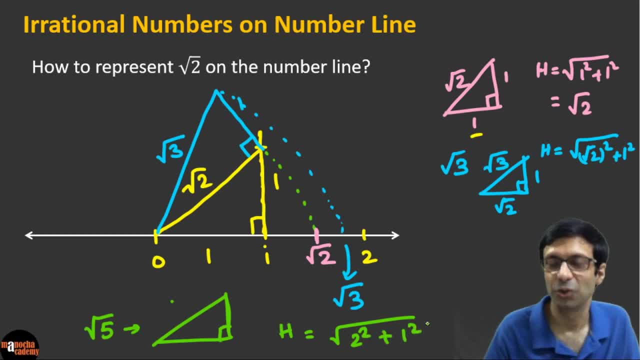 it's 2 square plus 1 square, right. So our sides are going to be 2 and 1, because 2 square plus 1 square is 5.. So that's a simple way to get the right. So again, we use another triangle, So the 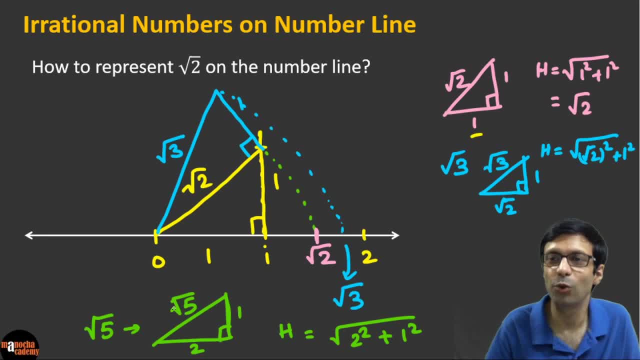 main thing is you need to decide your triangle and write it in this square root form and decide the length of your sides. So now we'll take the sides of length 2 and 1, and so I'm sure you guys can do this yourself, right? So please remember this important trick of how to represent. 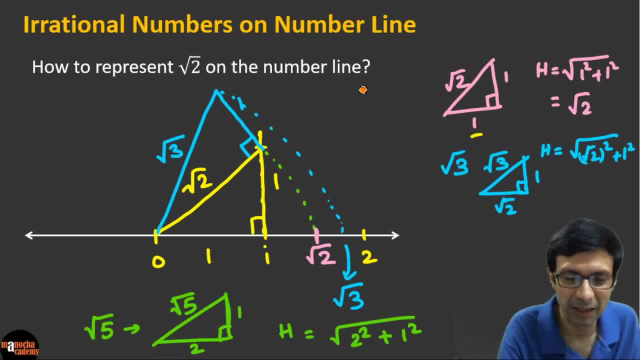 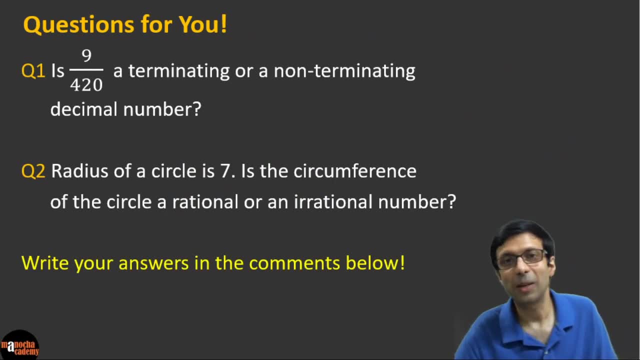 irrational numbers on the number line. okay, And this is a very important thing, and sometimes you get this question in your tests. All right, guys, and now I have some interesting questions for you to solve as your homework. So here are two questions. So the first question is: is 9 by 42? 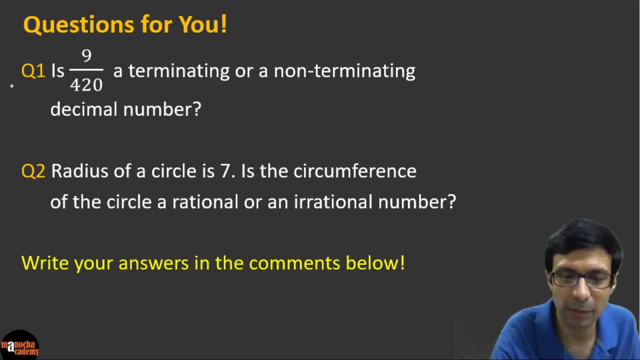 a terminating or a non-terminating decimal number right, So remember. one hint is: rather than a non-terminating decimal number, right, So remember. one hint is: rather than a non-terminating decimal number, right, So remember. one hint is: rather than using the calculator or solving, I taught 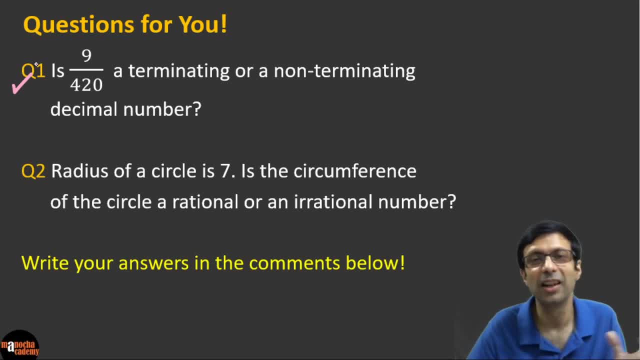 you a shortcut trick so you can use the rule that we learned to decide if this number is terminating or non-terminating. So that's my hint, but go ahead and take a look at the fraction carefully and solve this question. And there's another interesting, the second question for you. 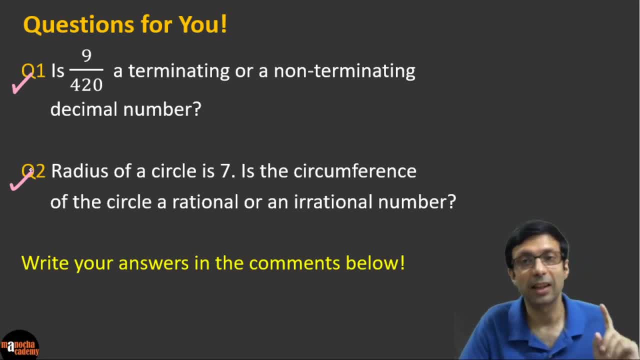 that if the radius of a circle is 7, is the circumference of a circle of the circle a rational or an irrational numbers? So these are your homework question, guys, and I want you to try these yourself and do write your answers in the comments below. I'm looking forward to 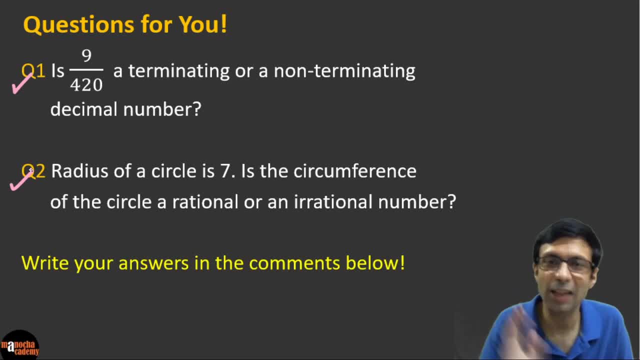 reading your answers and I promise you I'll reply to them as soon as possible, For the other live classes also. I've seen your answers and I'm replying to them as soon as I can. So go ahead and try these homework questions and do write your answers in the comments below. Okay, and guys, we 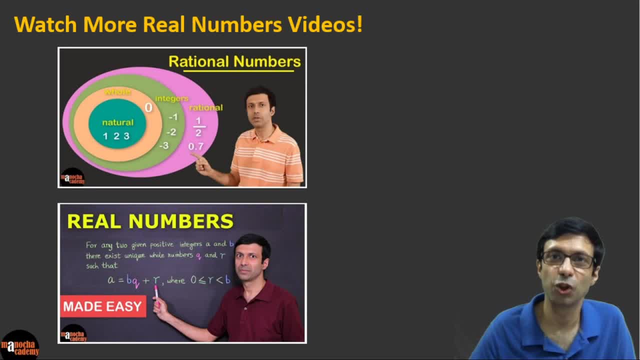 have some more real number videos on our YouTube channel. So do subscribe to our YouTube channel and do check out these videos. So this one is particularly useful for class 9 and for even for class 7 and 8, you know. So this video: 7,, 8 and 9th class can watch this video and this video is 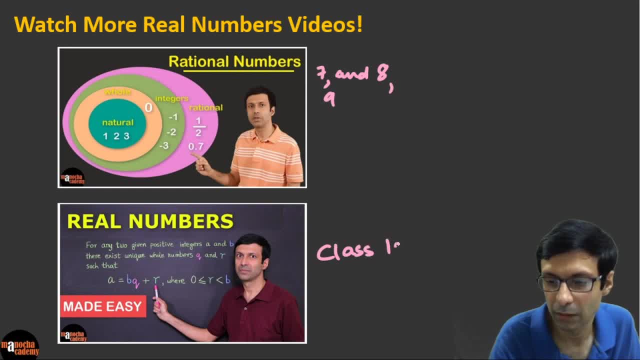 mainly for the class 10.. Right, so this. so we have this video on the rational numbers, which is mainly for classes 7, 8 and 9.. Right, and this real number video is for class 10.. So guys do watch these videos. I'll try to put the